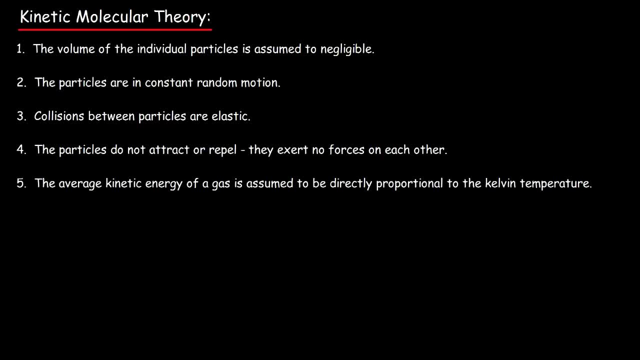 five facts. these are assumptions that describe the behavior of an ideal gas, which a real gas can deviate from such behavior. So the first assumption: the volume of the individual particles is assumed to be negligible, and for an ideal gas that's it's not important. So let's say, if you have a very large container, 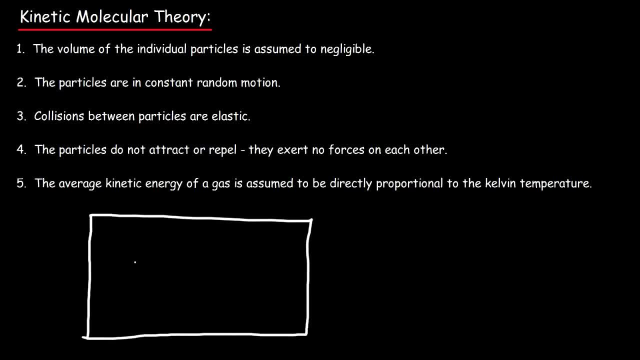 the gas particle is very, very small that the volume of that particular gas particle is negligible compared to the distance between gas particles. So the volume of the actual particles are so small that we don't have to worry about it. it's negligible. Now, for a real gas, that volume may be significant. 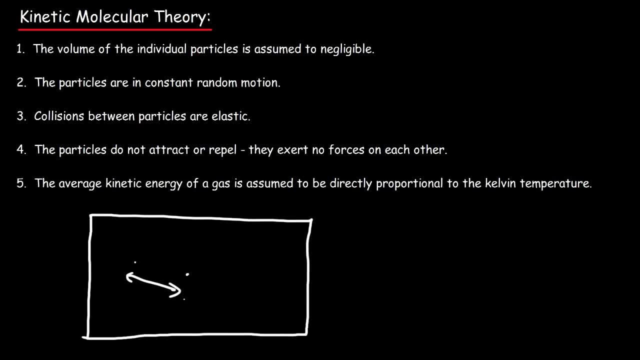 depending on the size of the gas. Some gas particles are bigger than others, and so the identity of the gas, the size that it has, can play a role in the pressure volume relationship of a real gas, For instance. according to Boyle's Law, if you increase the volume, the pressure will. 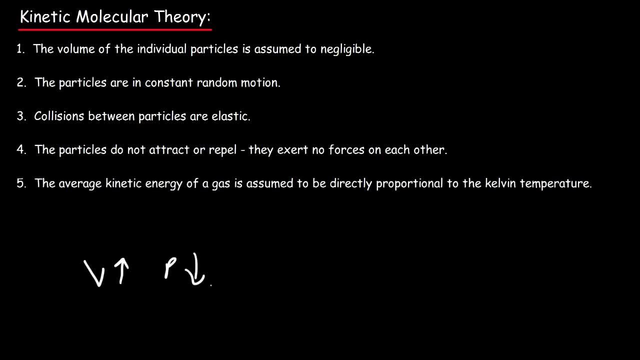 decrease. For an ideal gas, if you double the volume, the pressure will decrease by a factor of two. For a real gas, if you double the volume, the pressure will decrease, but it may not exactly be by a factor of two. It may decrease by 1.95, by 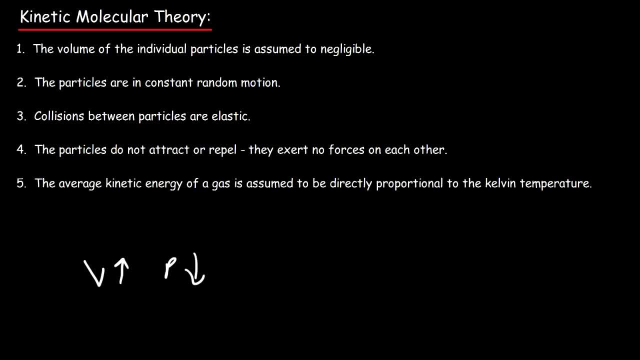 1.9 or 1.7 and each real gas will behave slightly differently. But for an ideal gas, if you double the volume, the pressure will decrease by a factor of two. But for a real gas it will deviate from that value because the 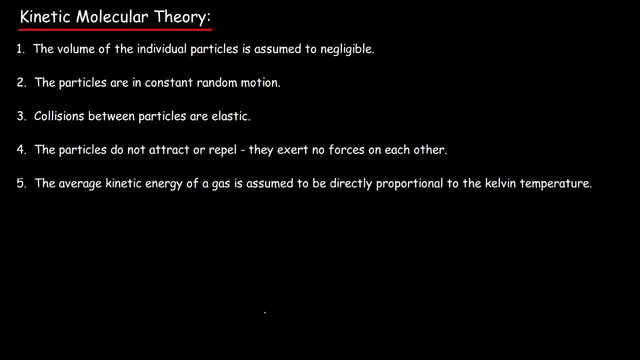 actual gas particles do take up space, But for an ideal gas we assume that such volume is negligible. Now the second assumption is that particles are in constant random motion, and for the most part this is pretty true. As long as the temperature is above absolute zero, the gas particles will be. 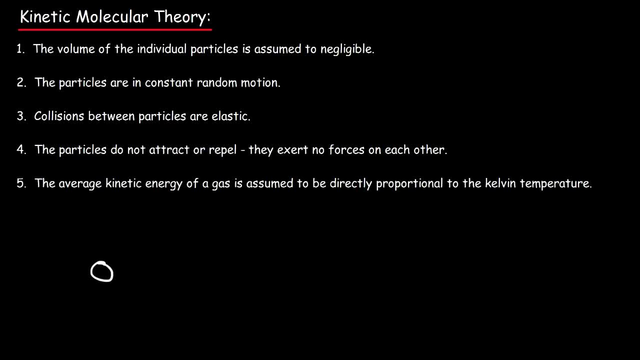 in motion. They're not going to just be sitting there and not moving. They're constantly moving and they move in straight lines. However, the motion is random. Let's say, for example, if you place a gas particle inside a test tube, It's not going to cruise directly straight, Rather, what's going to happen? 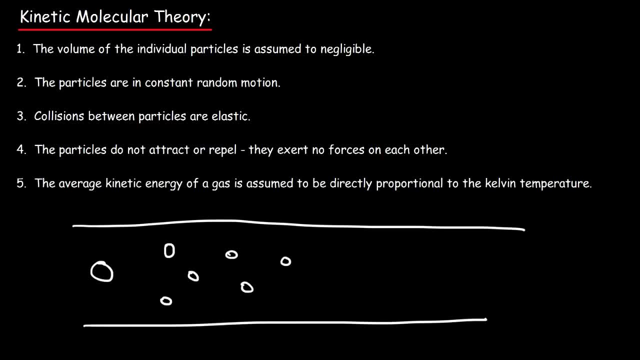 is because there's so many other molecules in its way, it's going to collide with these molecules and so it's going to constantly bounce around with the walls of the container and with the molecules in what appears to be a random motion, So it doesn't just go straight. Imagine if 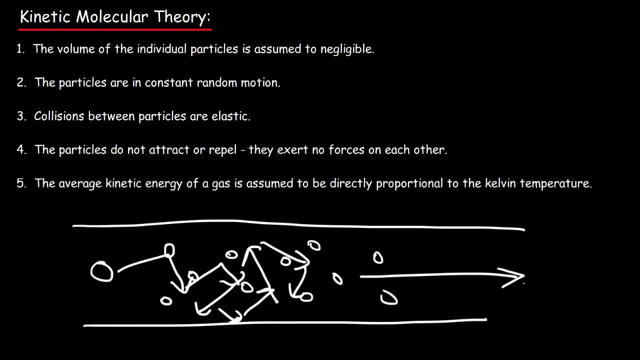 you're trying to hit a ball. Let's say you're playing pool and there's like a thousand other balls on the table and you're trying to hit a ball straight Because there's so many balls in the table. it's going to be very difficult. 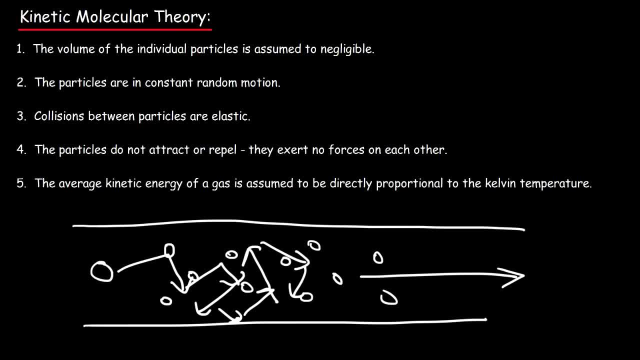 for you to hit it straight, It's gonna knock another ball. It's going to bounce around in different directions. Now in this test tube you have billions and billions of other gas particles, and for this gas particle to go straight it's not going to happen. So, because there's so 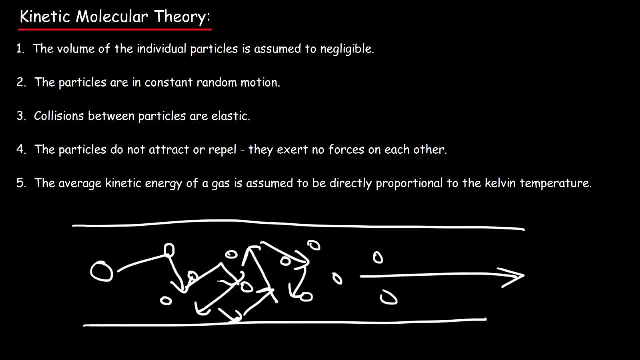 many other gas particles in its way. the motion will appear to be random. It's constantly going to be bouncing up and down as it makes its way through the test tube. Now the collisions between gas particles are elastic. An elastic collision means that kinetic energy is conserved. In an inelastic collision, kinetic energy is not. 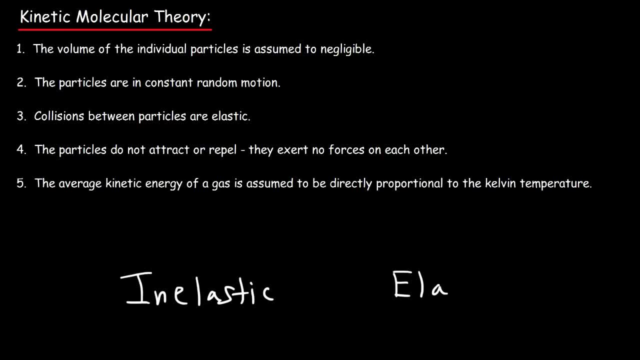 conserved, You have loss of energy. What we have is an elastic collision where kinetic energy is conserved. By the way, momentum, which is mass times velocity, is conserved for any collision, but for an elastic collision the kinetic energy is. 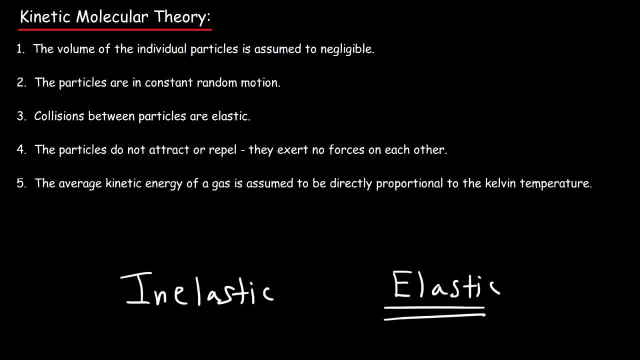 conserved. And. And when I mean kinetic energy, I mean the total kinetic energy of the system, not necessarily the kinetic energy of one particle, Because one particle could transfer its energy to another particle. When you have billions of particles, the total sum remains constant. 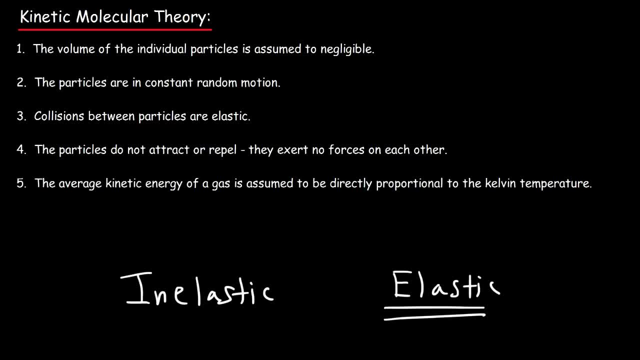 So we could say the collisions are elastic, There's no loss of kinetic energy. Now number four: the particles do not attract or repel. They exert no forces on each other, And this is true for an ideal gas. However, for real gases they do exert attractive and repulsive forces. 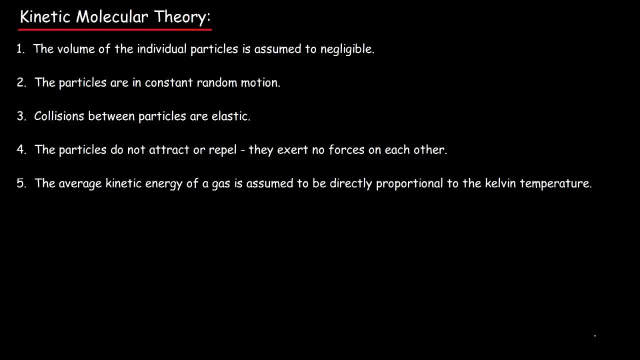 So, for example, let's use a polar gas like ammonia. Nitrogen is more electronegative than hydrogen, So therefore it bears a partial negative charge, And hydrogen is more electronegative than hydrogen, So therefore it bears a partial positive charge. 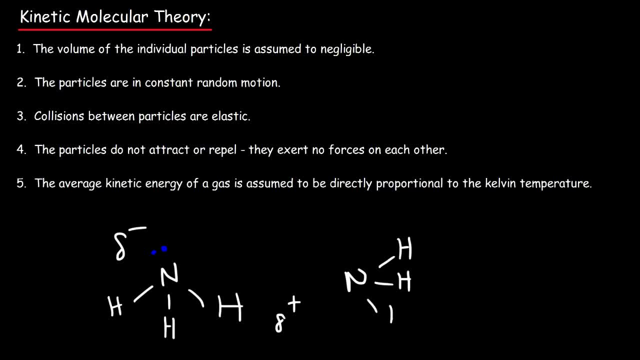 So when you have two ammonia molecules next to each other, the nitrogen of one molecule is going to be attracted to the hydrogen of another ammonia molecule, Because opposites attract. The hydrogen has a partial positive charge, The nitrogen has a partial negative charge. 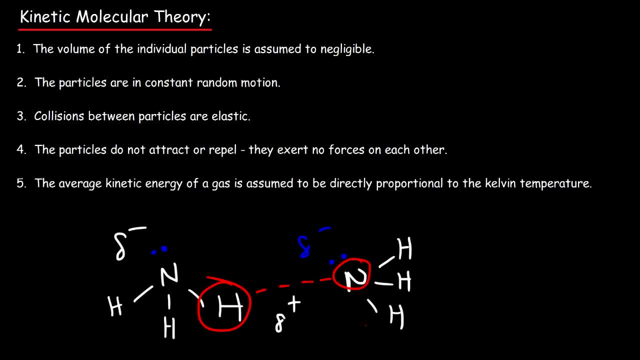 And so it's going to have an attractive force between them. So the hydrogen has a partial positive charge, The nitrogen has a partial negative charge. Now this nitrogen atom is repelled by the other nitrogen atom because they both have like charges: They're both partially negative. 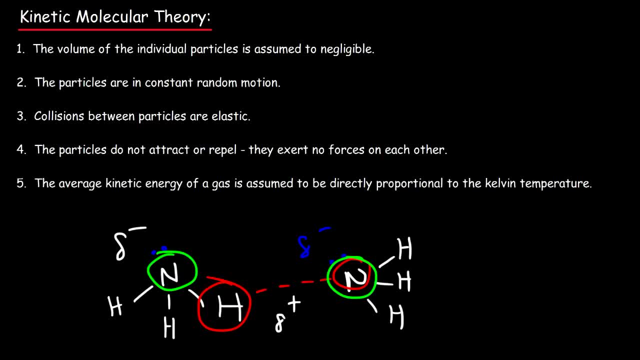 And so those two atoms will repel each other. And so whenever you have a polar gas, it tends to deviate from the behavior of an ideal gas. because there's forces between these molecules, They can attract or repel each other, But an ideal gas 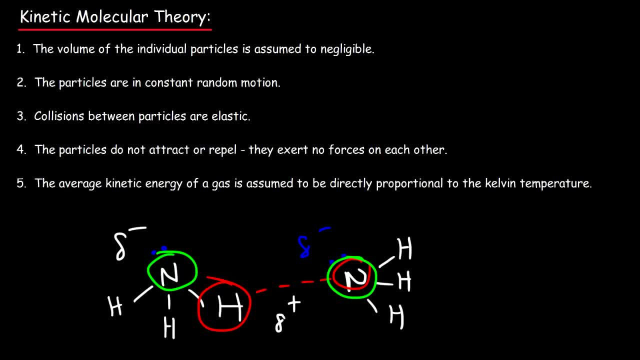 It's assumed to have no such forces. So the lesson to be learned from it is this: Polar gases tend to behave less ideally than nonpolar gases. Polar gases have intermolecular forces like dipole interactions and hydrogen bonds. Nonpolar gases, they only have weak London dispersion forces. 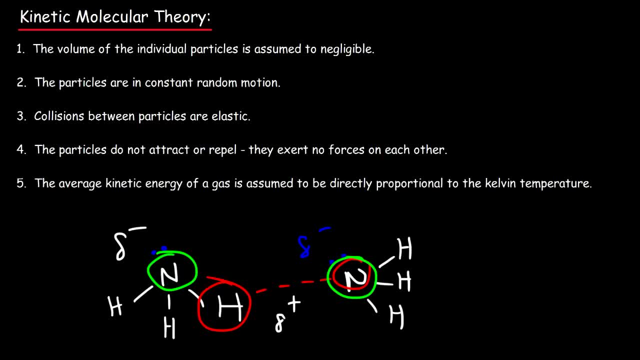 And so nonpolar gases tend to behave more ideally. So make sure you keep that in mind. Now the last statement. the average kinetic energy of a gas is assumed to be directly proportional to the Kelvin temperature, And this is true. Gases that exist at a higher temperature tend to be moving faster. 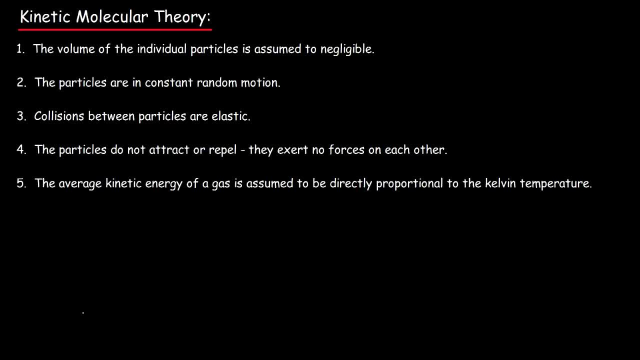 And as a result they have more kinetic energy. The average kinetic energy Of a gas is equal to three over two RT. It's directly proportional to the temperature. So if you increase the Kelvin temperature, the average kinetic energy of a gas increases. 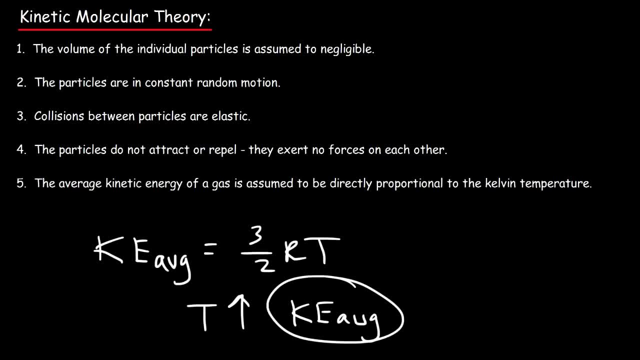 Now, this is not the kinetic energy of a single gas particle. Rather, it's the kinetic energy of a collection of gas particles, billions of gas particles together, And so when you average out the energies of billions of gas particles, you'll find that 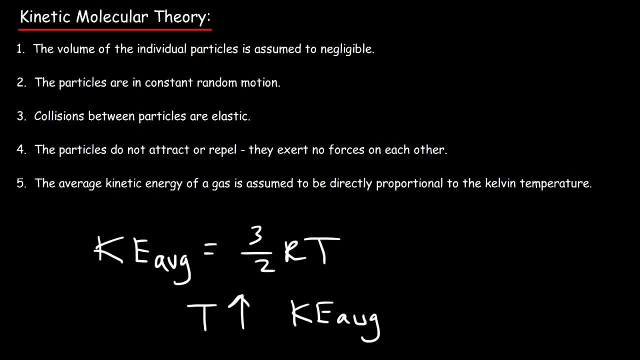 the kinetic energy is based on the temperature of the whole sample. If you're just looking at one individual particle, then the kinetic energy of that individual particle is dependent on the mass of the particle and the speed. But that's just for one particle. 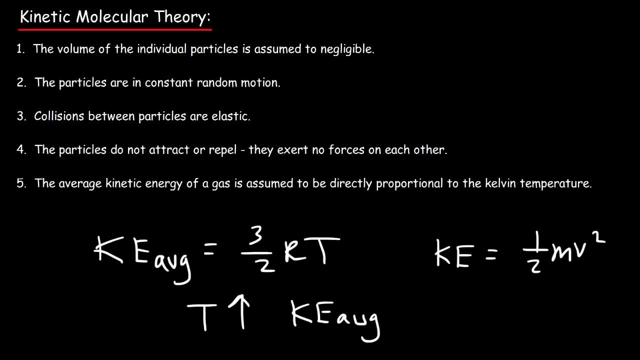 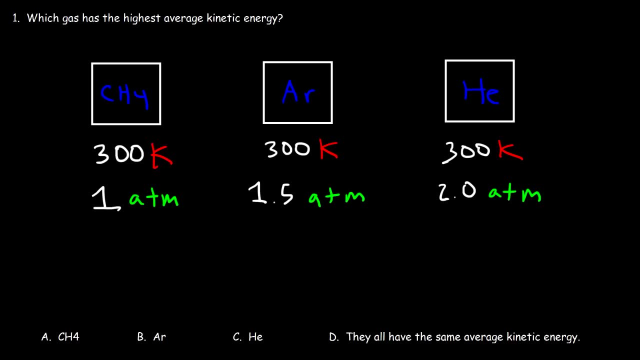 When you have billions of particles colliding with each other, it's only dependent on its temperature, So make sure you keep that in mind. So, keyword average: So you're dealing with a large number of gas particles. Now let's work on some multiple choice practice problems. 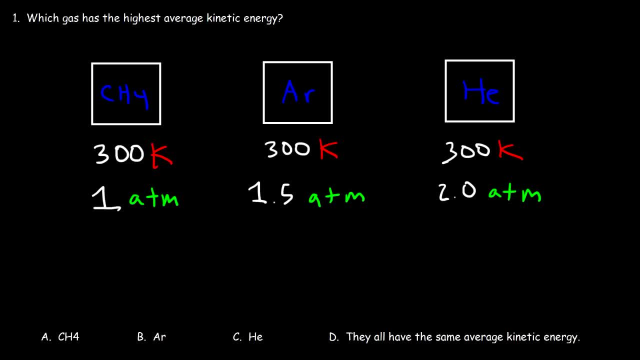 Which gas has the highest average kinetic energy? Is it going to be methane, argon or helium? We're given the temperature and the pressure of each gas And the size of the container is the same, so they all have the same volume. 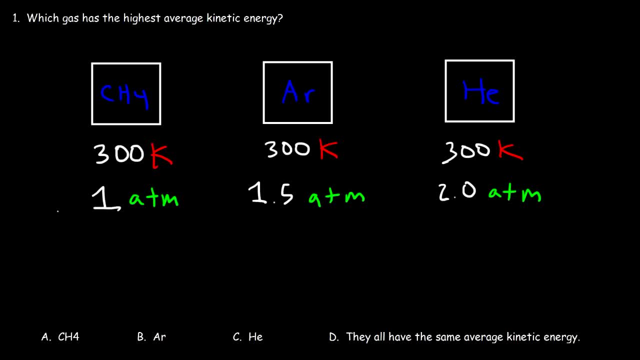 The pressures they vary. So is it going to be the one of the lowest, Methane, Or the one with the highest pressure, helium? Now, as was mentioned before, the average kinetic energy is proportional to the Kelvin temperature, And since the Kelvin temperature for each sample of gas is the same, then that means 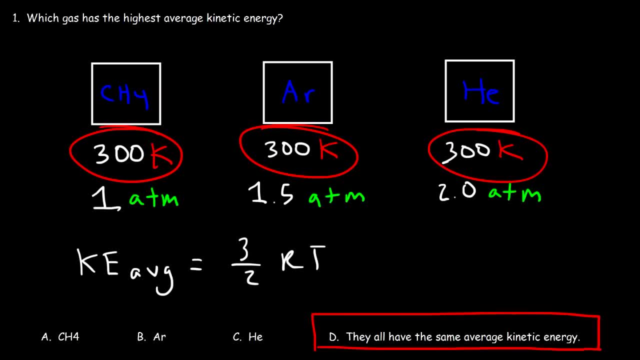 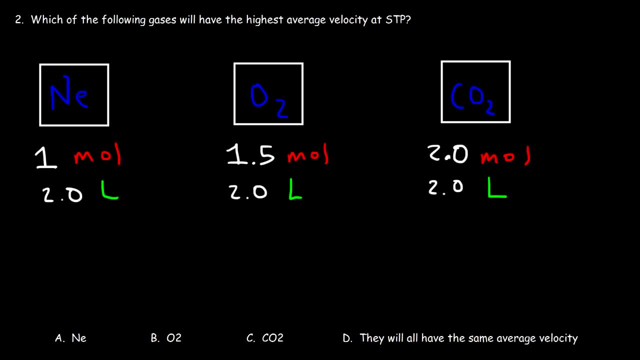 that they all have the same average kinetic energy. So D is the right answer. Now what about this one? Which of the following gases will have the highest average velocity at STP, standard temperature and pressure? So keep in mind: at STP the temperature is 0 Celsius or 273 Kelvin, and the pressure 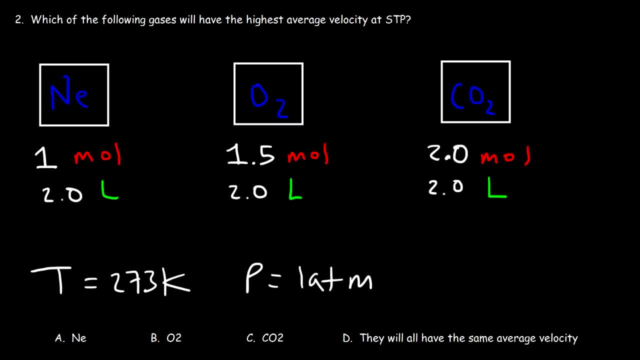 is 1 atm. So these conditions apply to each gas. So do you think the answer is going to be A, B, C or D? Well, We know that the average velocity represented by the root-mean-square velocity formula is equal to the square root of 3 RT divided by the molar mass of the gas. 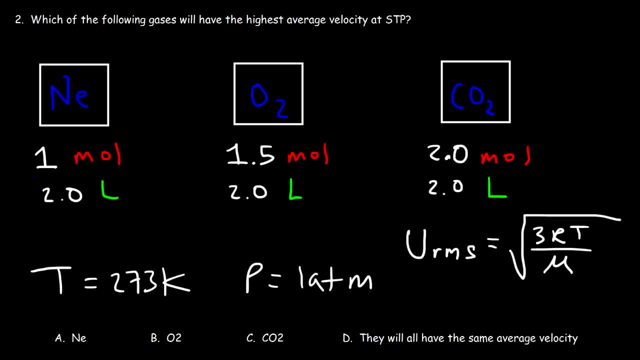 So the velocity doesn't depend on the number of moles or the volume of the container, And it doesn't depend on the pressure within the container. It depends on two things: The temperature and the molar mass. Now, the temperature is the same. 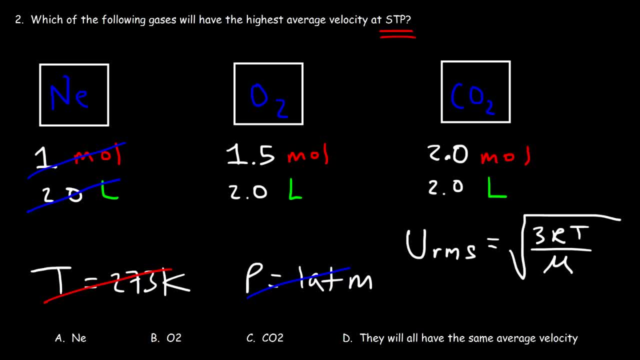 Every gas listed here is at STP, So the only thing that's different is the molar mass. What you need to understand is that heavy gases move slower and lighter gases move faster, So we're going to find out which of these gases has the lowest molecular weight or molar. 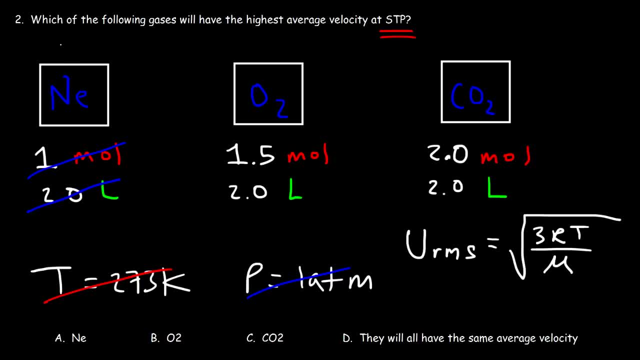 mass. According to the periodic table, neon has an atomic mass of 20.. Oxygen is going to be 16 times 2.. So we're going to find out which of these gases has the lowest molecular weight or molar mass. Oxygen is going to be 16 times 2.. 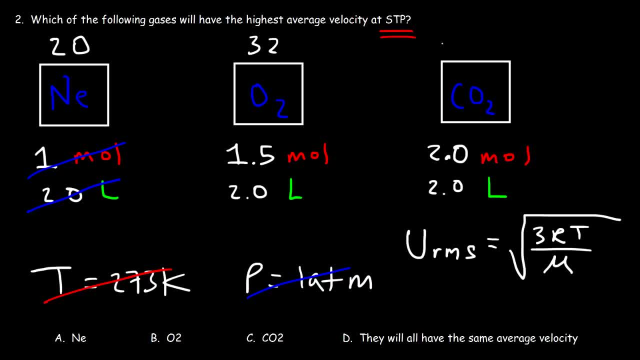 So that's 32.. And CO2, that's 12 plus 16 times 2, which is about 44. So neon is the lightest gas molecule, Which means it's going to have the highest average velocity. So A is the right answer. 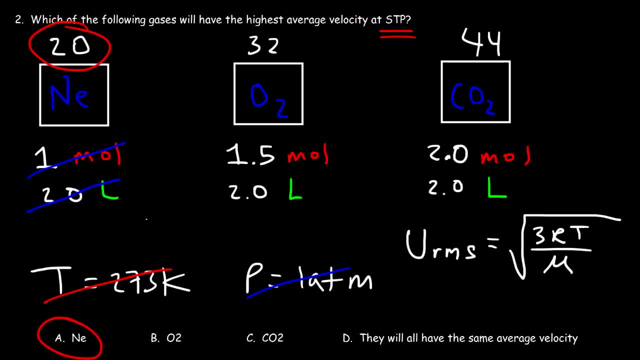 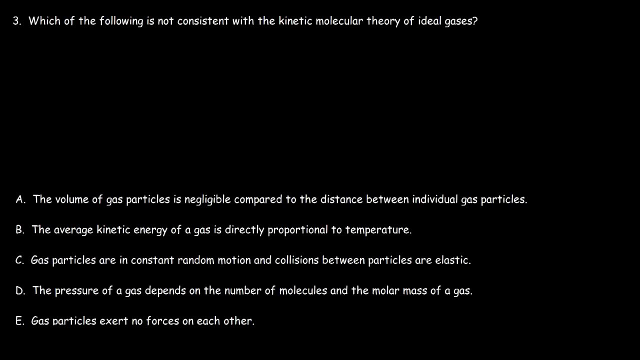 So, for average velocity, here's what you need to take, Or here's what you need to keep in mind. As the molar mass of the gas increases, the average velocity will decrease. Right as the temperature increases, the average velocity will increase as well. Let's: 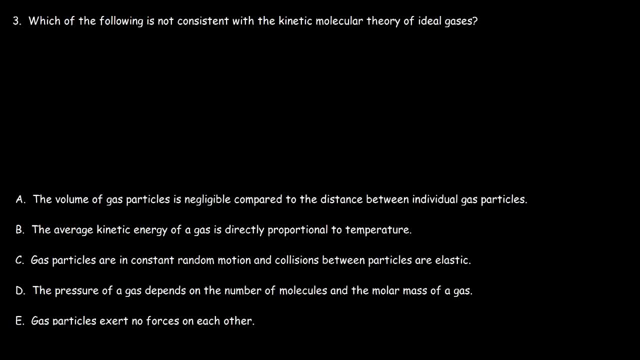 move on to number three. Which of the following is not consistent with the kinetic molecular theory of ideal gases? So let's go through each one. The volume of gas particles is negligible compared to the distance between individual gas particles. Is that true or false? Is that a statement that's found in the kinetic 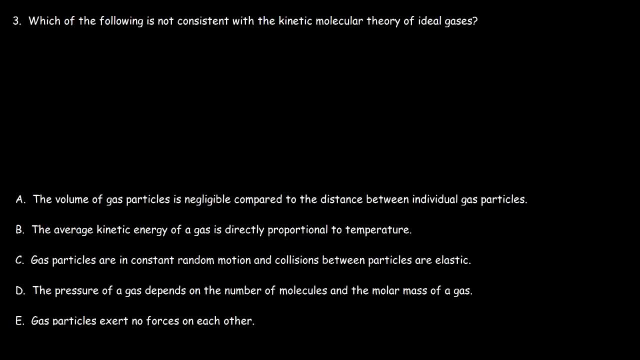 molecular theory of gases. A is a true statement B: the average kinetic energy of a gas is directly proportional to temperature. That's true as well. It's directly proportional to the Kelvin temperature, not the Celsius or Fahrenheit temperature. C gas particles are in constant random motion and 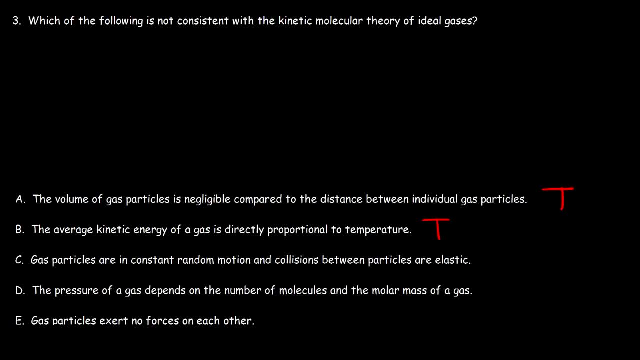 collisions between particles are elastic. C is true, The gas particles are always moving as long as the temperature is above absolute zero, and the collisions are elastic where the total kinetic energy is conserved. D- the pressure of a gas depends on the number. 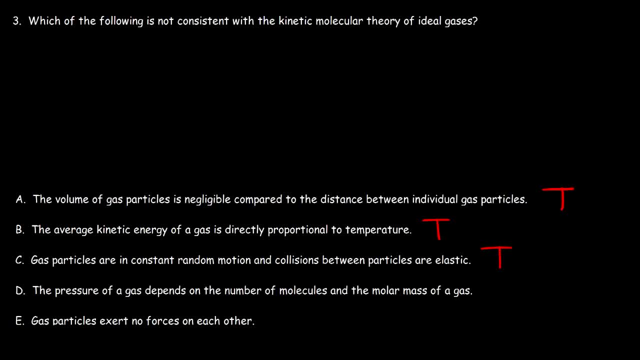 of molecules and the molar mass of a gas. Now D is not part of the kinetic molecular theory of gases. The first part of D is true. The pressure does depend on the number of molecules. however, it does not depend on the molar mass of a gas. So 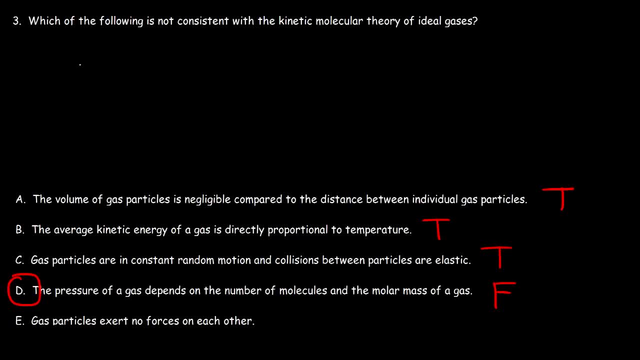 D is a false statement, which means this is the answer Based on this equation. if you solve for P, the pressure of a gas depends on N, which is the moles of the gas, particles And moles is proportional to the number of molecules. so that's why. 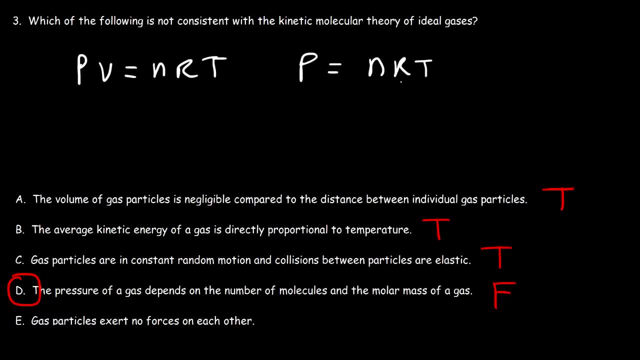 that part is true. The pressure depends on the temperature and also on the volume of the container. As you can see, molar mass is not part of this equation, so the pressure does not depend on the molar mass of gas And E is a true. 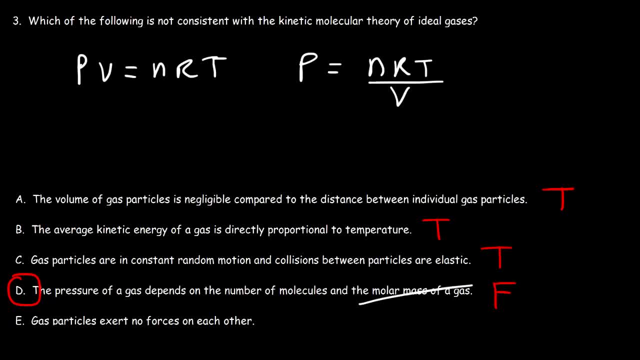 statement: Gas particles exert no forces on each other. Now this is true for ideal gases. A real gas may exert a force on another gas particle. They can attract other gas particles, they can repel them. It depends on the structure, the 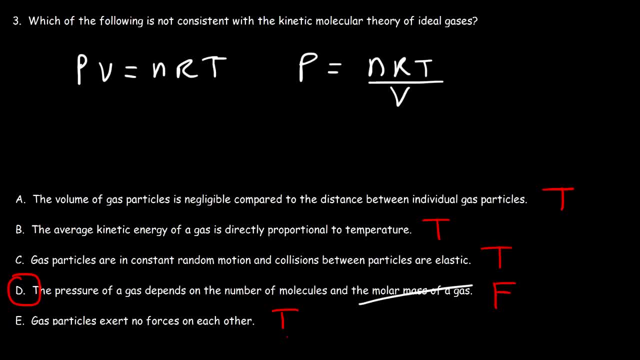 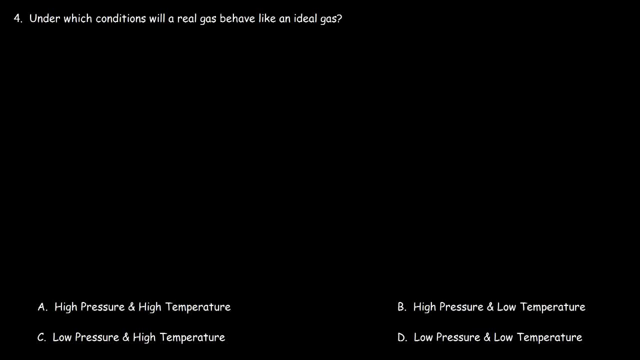 structure of the molecule and what it's made of. Number four: under which conditions will a real gas behave like an ideal gas? Is it at high pressure or at low pressure? And at high temperature or at low temperature? what would you say? 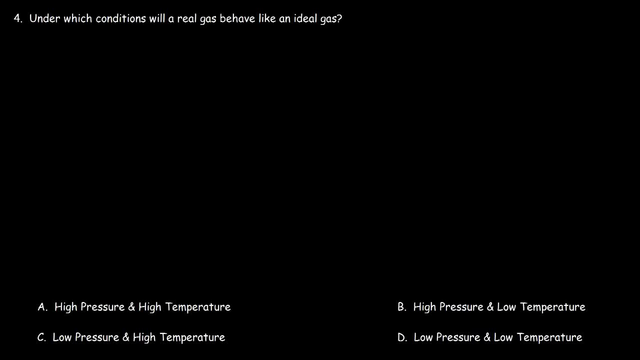 Now imagine if you have a liquid. if you decrease the temperature, will the liquid become a solid or will it turn into a gas? Something I like to use to explain this is a phase diagram, And if you haven't seen a phase diagram, it basically tells you where a solid, a liquid 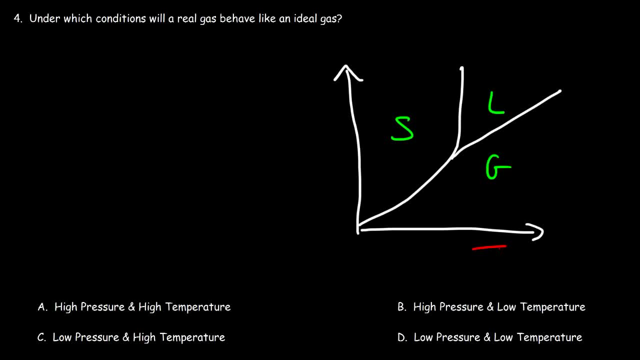 and a gas co-exist under conditions of temperature and pressure. So on the y-axis you have pressure, on the x-axis you have temperature. So let's start somewhere in the liquid phase. Okay, So if we decrease the temperature, that means we have to travel towards the left on the 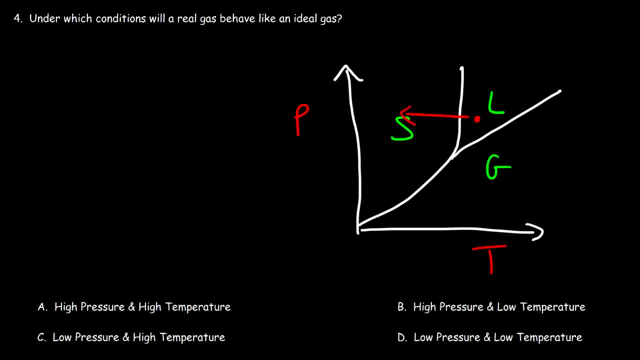 x-axis. If you decrease the temperature of a liquid, it's going to turn into a solid, So low temperatures do not favor the formation of a gas. If you put liquid water in the freezer, the temperature will decrease. It's going to turn into ice. 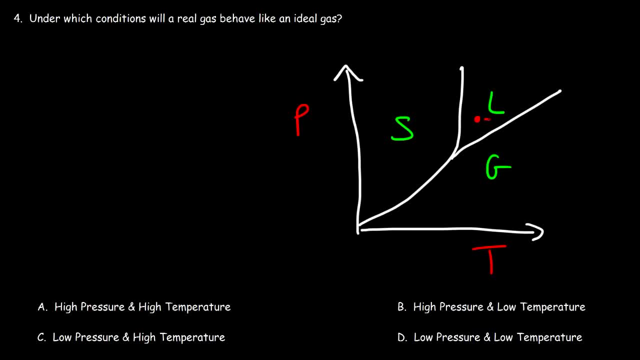 So you don't want that. Rather, if you increase the temperature, if you travel towards the right on the x-axis, the liquid will become a gas. If you take the liquid water and put it on a stove, it's going to vaporize into steam. 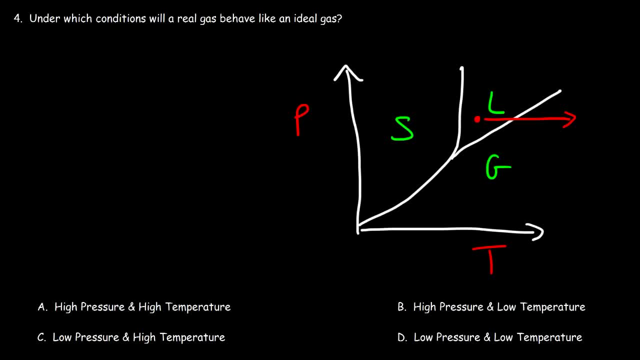 Thus a real gas will behave more like an ideal gas under conditions of high temperature and not low temperature. If you decrease the temperature, it will no longer be a gas. It's going to eventually turn into a solid, So high temperatures favor the formation of gases. 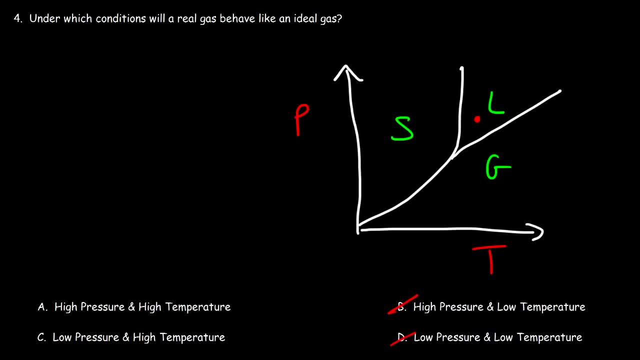 So we could eliminate answer choice B and D. Now, what conditions will favor the formation of a gas: High pressures or low pressures? Well, if we start from the same position, if we increase the pressure, that means if we travel towards the positive y-axis, it's not going to turn into a gas. 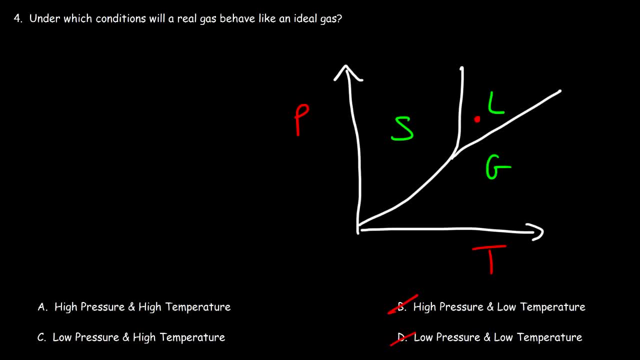 But if you decrease the pressure, Okay, The liquid will eventually become a gas. The best way to illustrate this is the boiling of water at different elevations. So let me draw a picture. So let's say this is a mountain And here we have a valley. 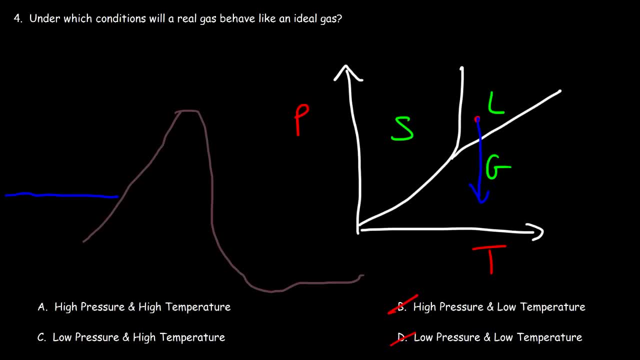 Let's say this is sea level. At sea level the atmospheric pressure is 1 atm. On the top of a mountain It might be less, Maybe like 0.6 or 0.7 atm. Atmospheric pressure decreases with increase in elevation. And at a valley the pressure is going to be higher, Maybe like 1.2 or 1.3 atm. The boiling point of water at 1 atm is about 100 degrees Celsius. At 0.7 atm it's going to be less than 100.. 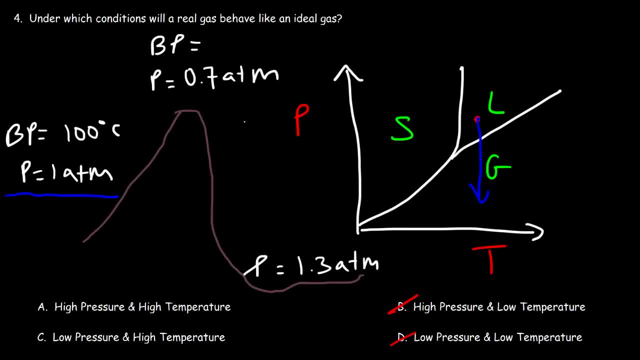 So I'm going to just pick a number that's less than 100.. It may not be the exact same number, It may not be the exact number that corresponds to this pressure, But for illustrative purposes let's say it's like 85 or 86 degrees Celsius. 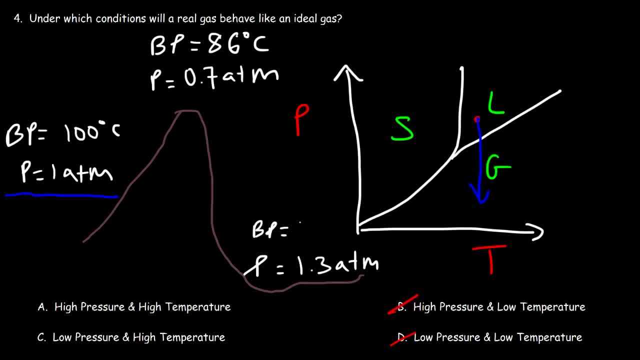 And at 1.3 atm, let's say it's about 108 or 109 degrees Celsius. But the point is that as the pressure increases, the boiling point of water increases, And so it's harder to boil water at high pressures. 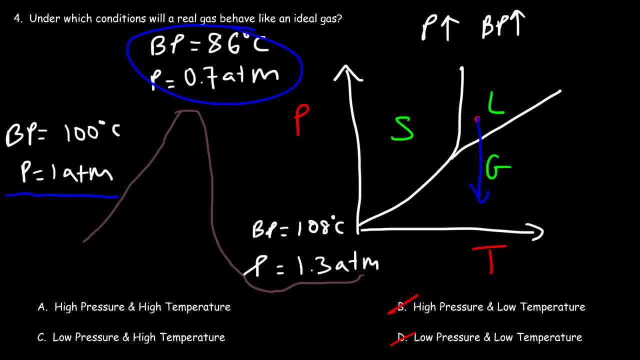 But it's easier to boil water at low pressures. Okay, So if you decrease the pressure, it's a lot easier for a liquid to enter the gas phase. because the boiling point has been reduced. The energy required to vaporize a liquid is not as high as before. 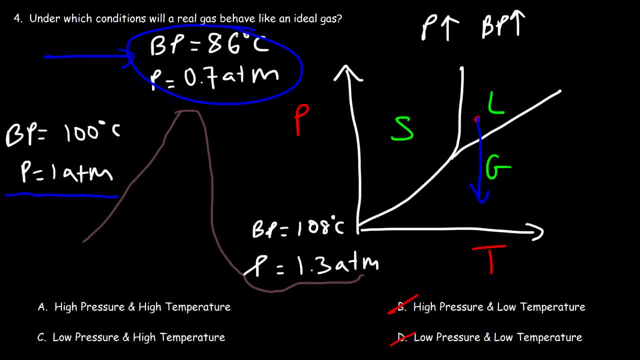 You only have to reach a temperature of 86 to boil water at, let's say, the top of a mountain rather than 100 at sea level. And so when you decrease the atmospheric pressure, you make it easier for the liquid to enter. 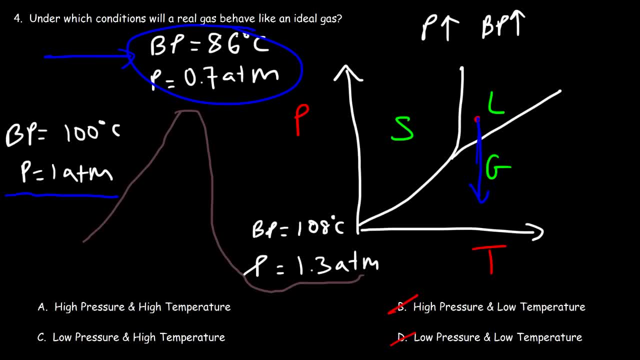 the gas phase, And so you're going to travel down on the phase diagram. So, therefore, if you decrease the pressure, a substance will behave more like a gas. If you increase the pressure, it can behave more like a solid or more like a liquid, depending. 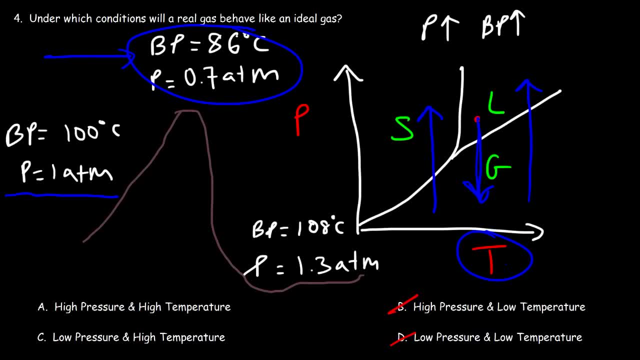 on where you are on the temperature axis. So a real gas will behave more like an ideal gas at low pressure. Okay, low pressure. so if you think of the location of the gas phase in this phase diagram, it exists towards the right, that is, towards high temperature, and it 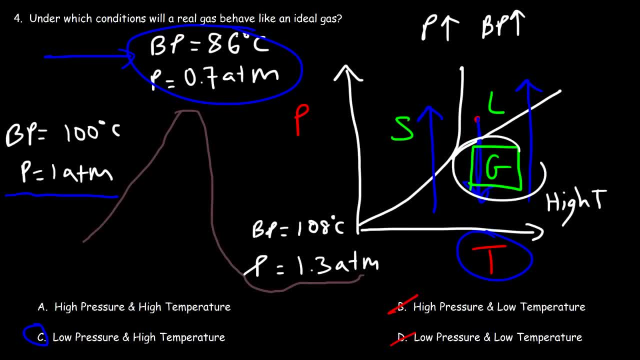 doesn't exist at the top of the graph. it exists at the bottom of the graph, so at low pressure. so gases tend to form under conditions of low pressure and high temperature. solids tend to form under conditions of low temperature and high pressure. liquids tend to form under conditions of relatively higher. 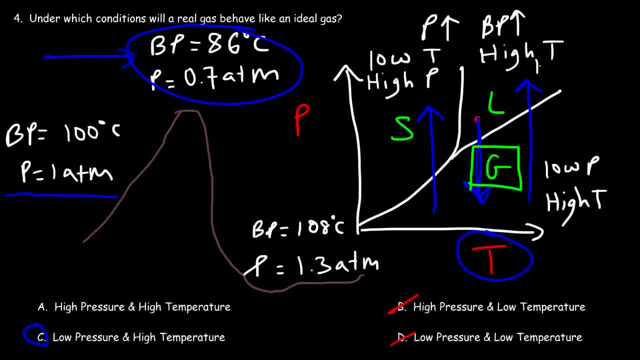 temperatures than solids, but higher pressures than gases. but the answer for this problem is C. so if you ever see a question like this, a real gas behave like an ideal gas under conditions of low pressure and high temperature. number five: which of the following real gases will best? 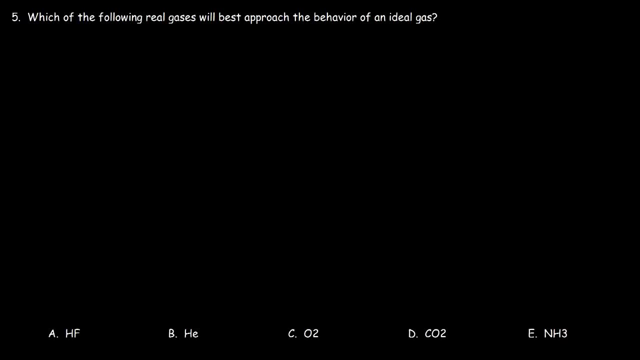 approach the behavior of an ideal gas. now, keep in mind what we said earlier: polar molecules will not behave like an ideal gas, but non polar molecules will behave more like an ideal gas. polar molecules tend to deviate from ideal gas behavior. so which molecules are polar and which ones are not? if you want to find out, if you need to review polar and 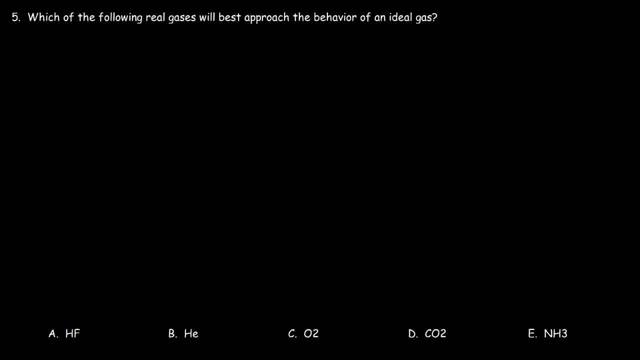 nonpolar molecules. you can search out a video that I've created on YouTube that can help you to distinguish it. but typically if a molecule has hydrogen bonds, it will be polar for the most part. so whenever you see H hydrogen directly bonded to one of these elements- nitrogen, oxygen or fluorine- then those bonds are. 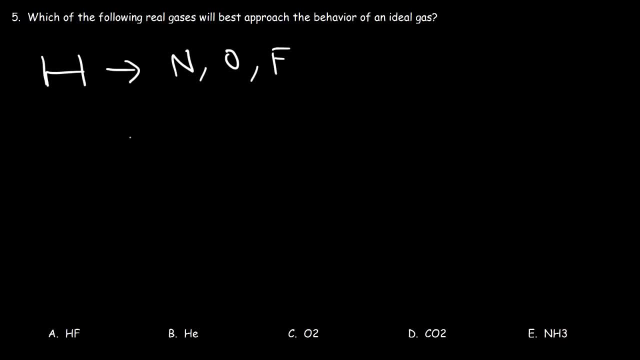 polar, So HF is a polar molecule. Fluorine is very electronegative and so it tends to pull the electrons toward itself. So as a result, fluorine acquires a partial negative charge and hydrogen acquires a partial positive charge. And so whenever you have a molecule where one side is partially positive and the other, 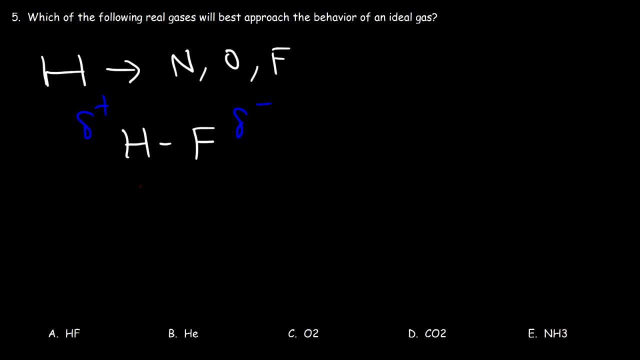 side is partially negative and if there's a net dipole moment, then the molecule is going to be polar. So HF is not going to behave like an ideal gas due to the forces that it will exert on other HF molecules. NH3 is another polar molecule. 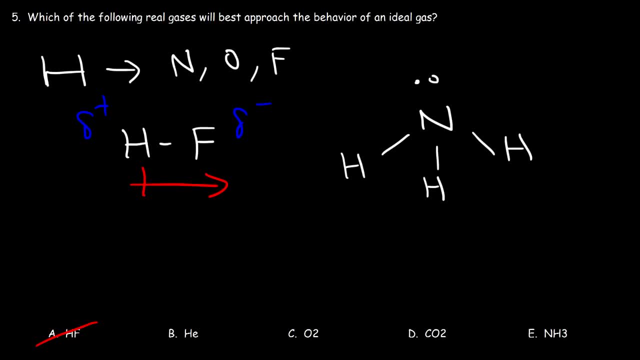 As you can see, we have hydrogen bonds between ammonia molecules, And so we can eliminate this one as well. It's not going to behave like an ideal gas. Now what about carbon dioxide? Is it polar or is it non-polar? Carbon dioxide has polar bonds. 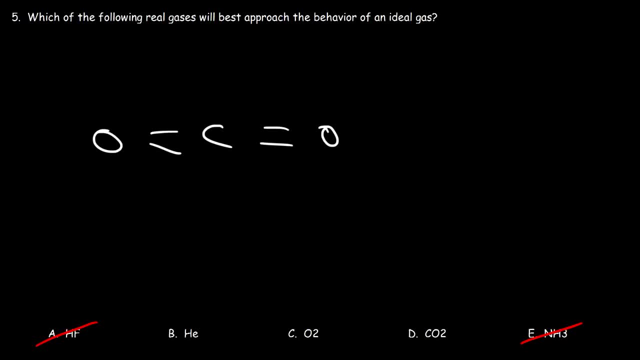 To determine if a bond is polar, you need to look at the difference in the electronegativity values. Carbon has an electronegativity value of 2.5 and oxygen is 3.5.. If you type in electronegativity, you're going to find that carbon dioxide has an electronegativity. 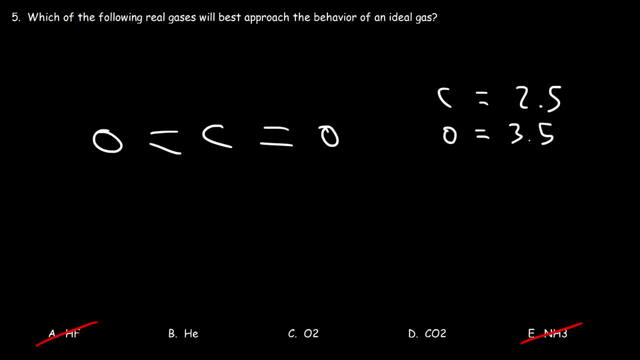 value of 2.5.. If you look at the electronegativity chart in Google Images, you can find these values. If the electronegativity difference is equal to or greater than 0.5, then the bond is polar. 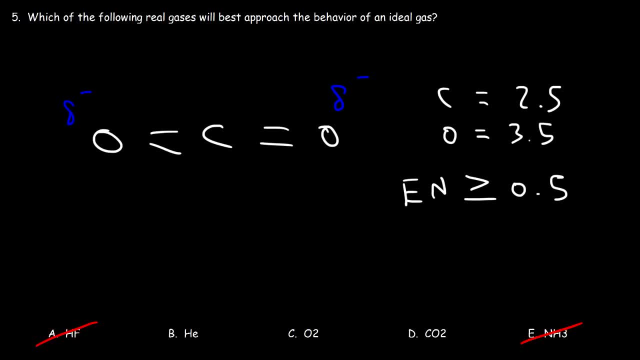 So oxygen carries a partial negative charge and carbon carries a partial positive charge. However, the dipole moments, which are arrows that you draw from a positive atom to a negative atom, notice that the arrows point in the opposite direction, And so the net dipole moment of CO2 is zero. 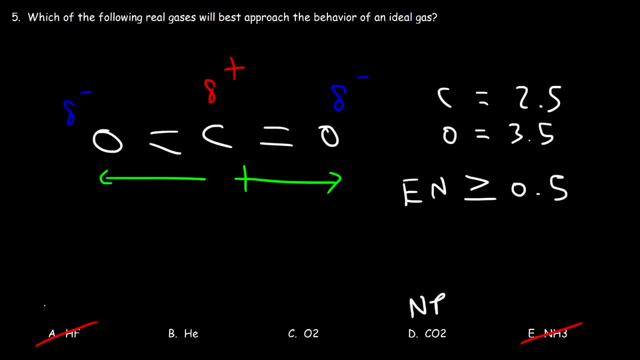 So CO2 is a non-polar molecule. HF and ammonia are polar molecules. Now, if you have an element or substance that's composed of just one element, it's always going to be non-polar. So the two oxygen atoms in an oxygen molecule are non-polar. 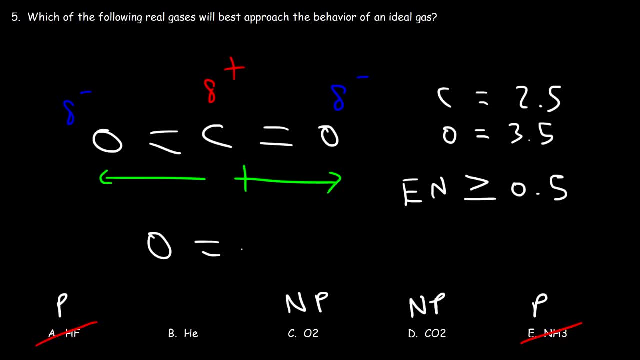 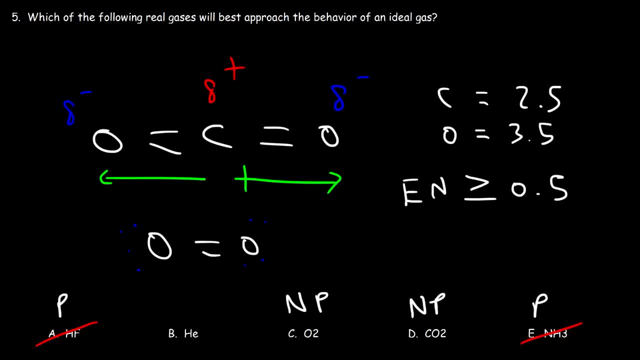 And so you're not going to have a positive atom and a negative atom. It's just not going to happen in this case. So the O2 molecule is non-polar And helium it's just an atom, It's electrically neutral. 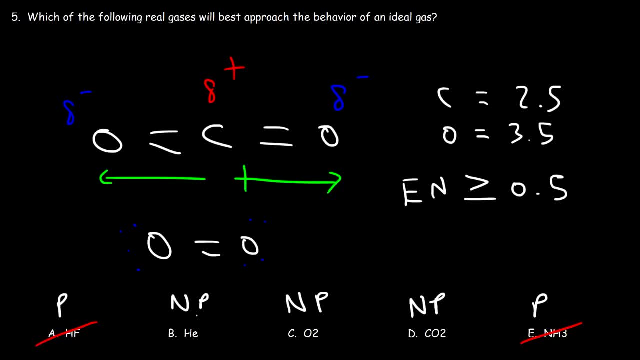 The electrons are distributed evenly around that atom, so it's going to be non-polar When the electrons are not distributed evenly in the case of HF, because fluorine pulls the electrons towards the right. that's why you have one side as negative and one side. as positive And so that uneven distribution of electrons creates a polar molecule. But in O2, the two atoms are the same, so the distribution of electrons are equal, which makes the molecule non-polar. So these three gases, helium, oxygen and CO2.. 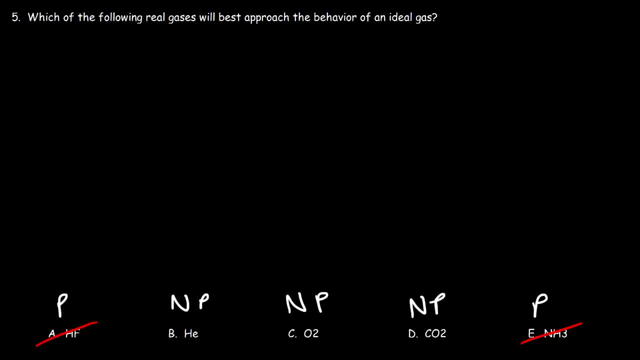 They will behave more ideally than HF or any stream. But among these three gas molecules, which one will behave most ideally compared to B, C and D? Now, the only type of intermolecular force that acts on a non-polar molecule are London. dispersion forces, And those forces depend on the molar mass of the molecule. As the molar mass of the molecule increases, the London dispersion forces will increase, And an ideal gas is one that does not have any forces that are exerted between the gas. particles. So therefore we want to reduce this as much as possible. The only way to do that is to decrease the molar mass And therefore we can decrease the London dispersion forces. So we need to identify which dispersion forces are the ideal gas. So we need to identify which dispersion forces are the ideal gas. We need to identify which non-polar gas molecule has the lowest molar mass. CO2 has a molar mass of 44.. O2 has a molar mass of 16 times 2.. It's 32 based on the periodic table, And helium is 4.. So helium has the lowest molar mass, So it has the lowest amount of intermolecular forces among helium atoms. Therefore it's going to behave most ideally. So we need to identify which non-polar gas molecule has the lowest molar mass. 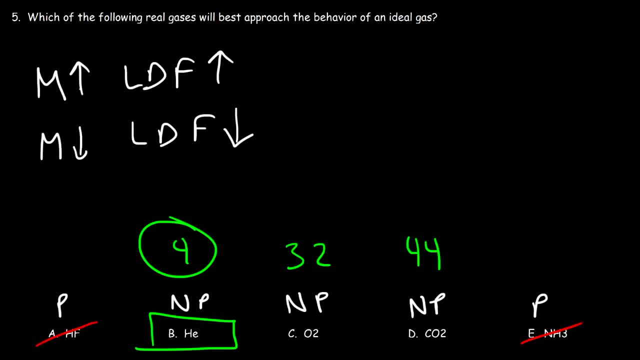 Now you can look at this problem from another perspective. Recall that one of the assumptions of the kinetic molecular theory of gases is that the volume of the gas particles has to be negligible, So a gas that has the least amount of volume will behave more ideally as well. 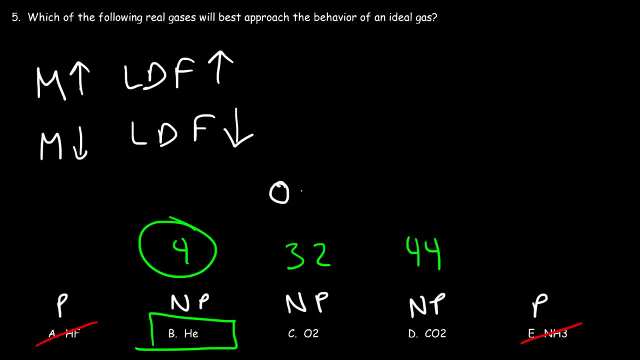 Now, if we look at the case of oxygen, oxygen is composed of two oxygen atoms. Carbon dioxide is composed of two oxygen atoms, Carbon dioxide is composed of two oxygen atoms And carbon dioxide is composed of three atoms And helium is composed of a single atom. 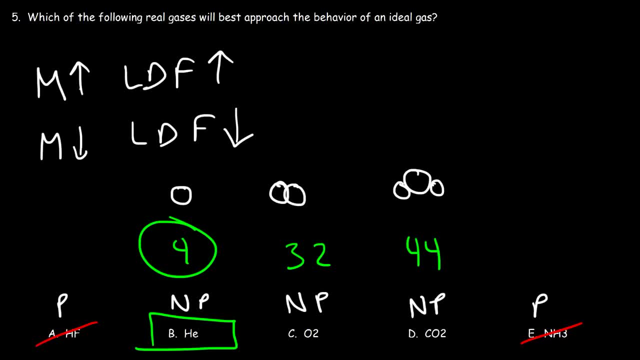 And helium is a lot smaller than oxygen or carbon, So therefore helium has the smallest volume, which is another reason why it behaves more ideally than O2 and CO2.. So the substance with the lowest molar mass tends to exert less forces. 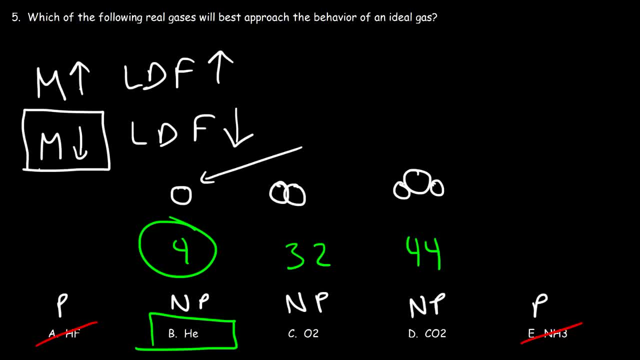 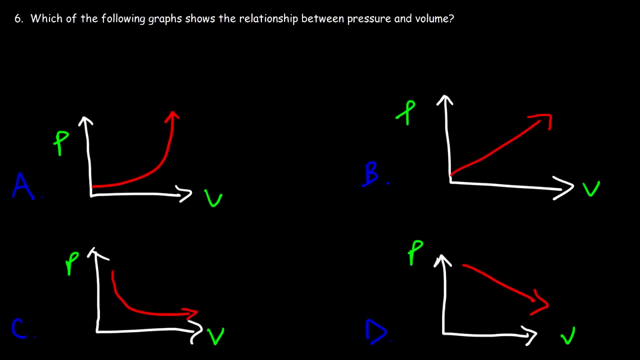 And at the same time, the substance with the lowest molar mass tends to exert less forces. the same time takes up less space or less volume, which makes it behave more ideally. so there's two reasons why substances would look with a small molar mass will behave ideally: less forces and less volume. number six, which of the 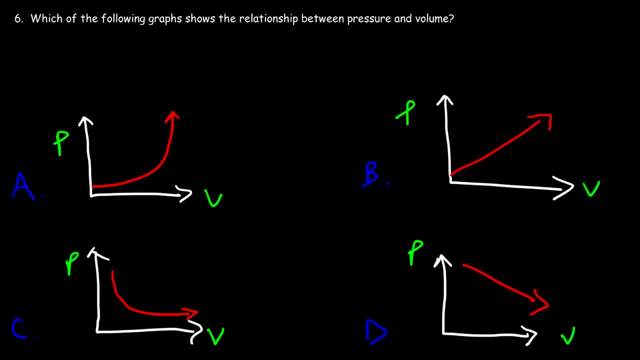 following graphs shows the relationship between pressure and volume. so think of for us which craft is associate with Boils law. increase the volume of the container. what happened to the press heurese of world's longest pressure would reduce. we have an inverse relationship, so that is not going to be. 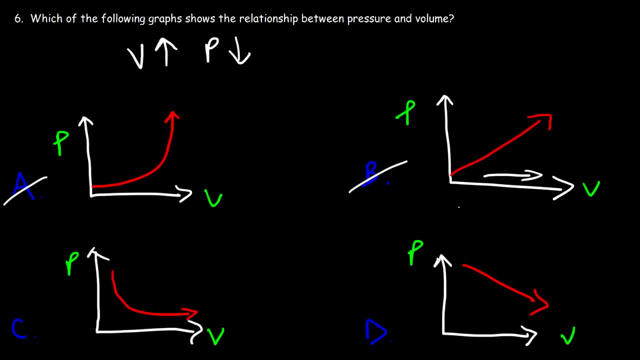 is not a, because as we increase the volume, as he movedtv right- the pressures increasing and so those two can be eliminated. is it gonna be sea or is it gonna be Res04? it's not gonna beat you, it's not gonna be d. the answer doctor and you have are fairly well right works. 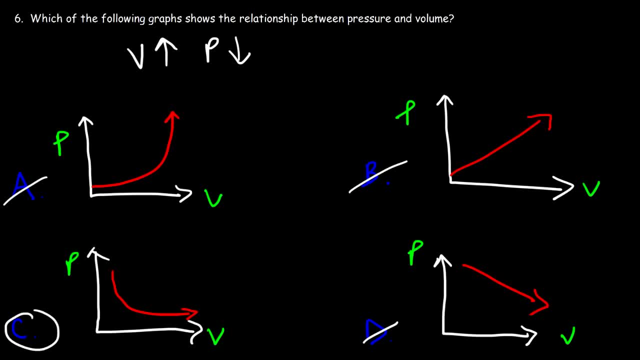 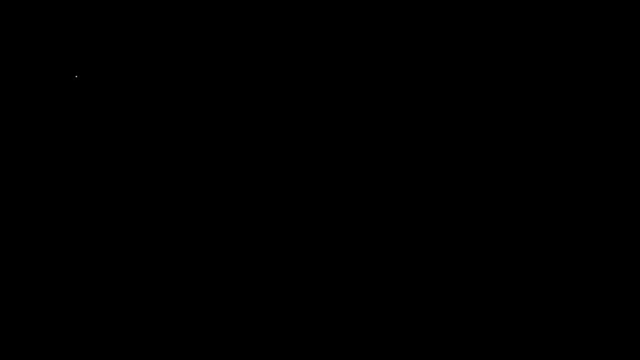 is C. There's only two graphs that you need to be familiar with. This is the graph of Boyle's law. It's a curved graph. It doesn't decrease at a linear rate. The other laws look like this. It's a straight line. So for Charles' law, if you increase the temperature, 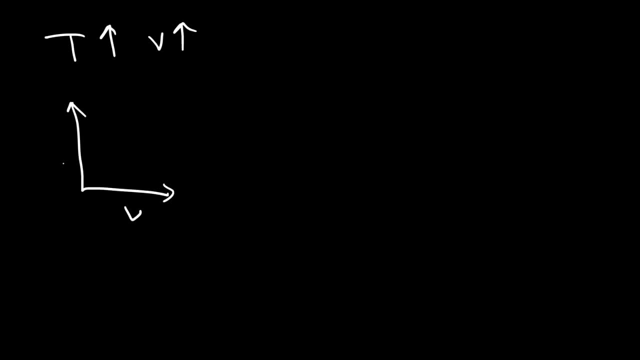 the volume will increase. So it has this shape. And then you have Gay-Lussac's law, where if you increase the temperature, the pressure will increase. It also has the same shape. And then, finally, Avogadro's law, where if you increase the moles, the volume will increase. 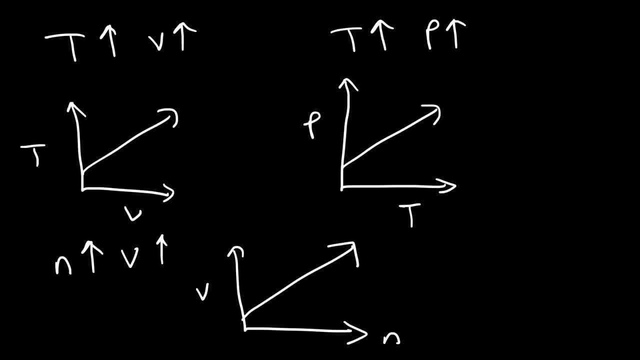 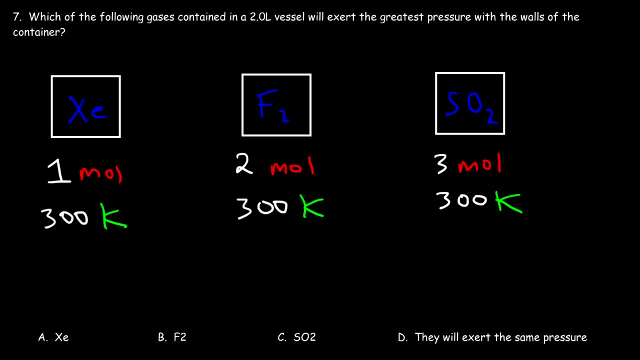 So here's N and here's V, Number seven. Which of the following gases contained in a two-liter vessel will exert the greatest pressure with the walls of the container? Is it going to be the sample of xenon gas, fluorine gas or sulfur dioxide gas? 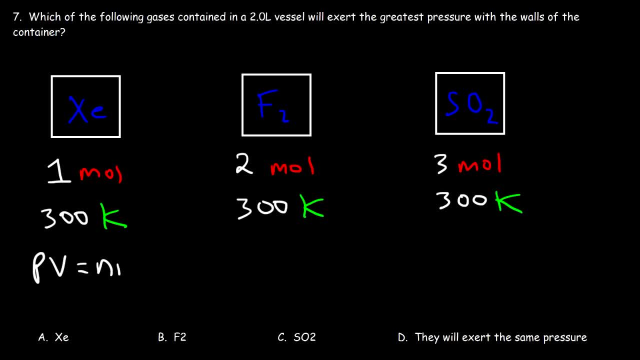 Now, going back to this equation, PV is equal to nRT. The pressure depends on the moles, the temperature and the volume. Now, the volume is the same, so we don't have to worry about that. The temperature is the same because each container is at 300 Kelvin, The only 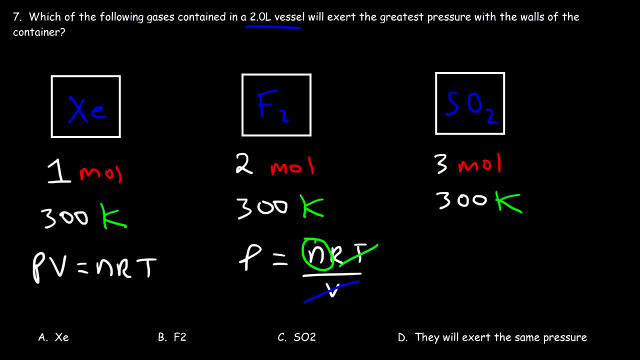 difference is the moles, And the pressure is proportional to the number of moles. If you increase the moles of gas within the container, the pressure will increase, And the reason why the pressure goes up is because if you have more molecules inside a container, there. 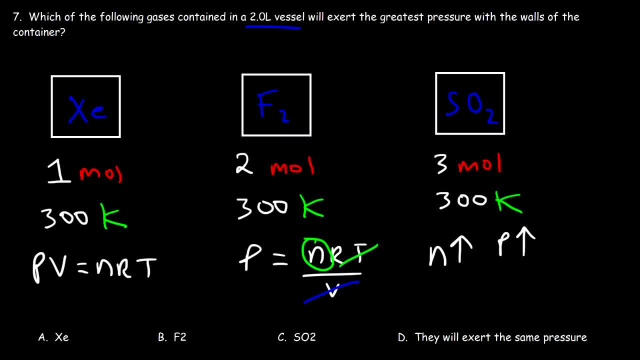 will be more collisions with the walls of the container And every collision exerts a force on that container And pressure is force per unit area. So if you increase the number of molecular collisions, the pressure will increase. And the reason why the pressure 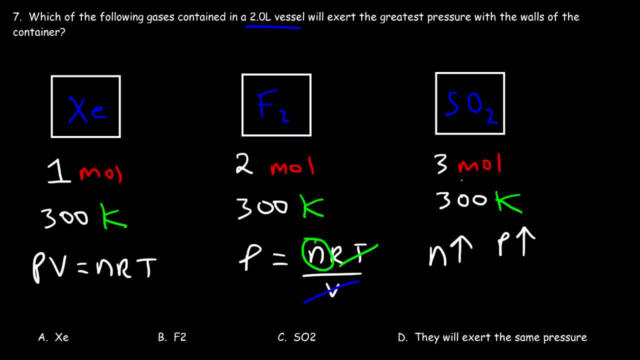 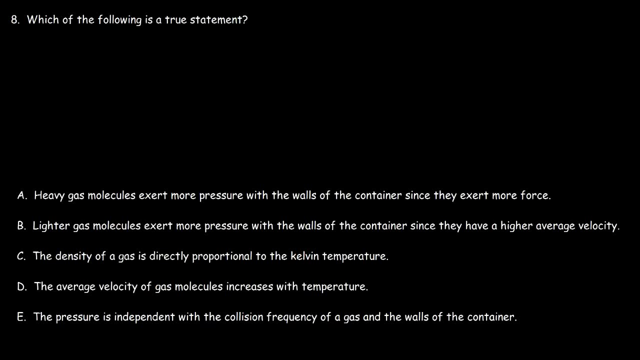 increases is probably because that the other guy had a higher pressure. The next one I said is that if one of the molecules goes under the complex and the center, peaceful, and so if the individual is less competitive enough at pulling 0 molecules from other decisions. 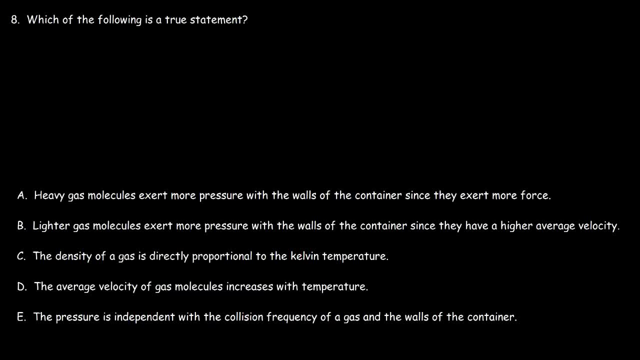 the pressure will increase. So therefore, the right answer is SO2, because we have the greatest quantity of molecules in that container. So C is the right answer because it has the highest number of moles. that true or false, now you might think a heavy object when it collides with 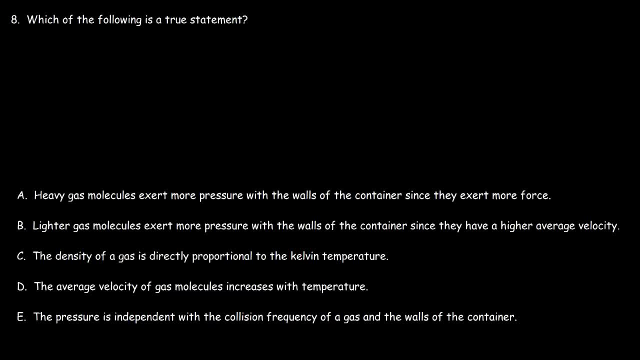 something might exert more force and, for the most part, if the speed is the same, that would be true. however, when you compare heavy gas molecules with light gas molecules, heavy gas molecules, even though they have more mass, they move more slowly, and lighter gas molecules, even though they have less mass, they 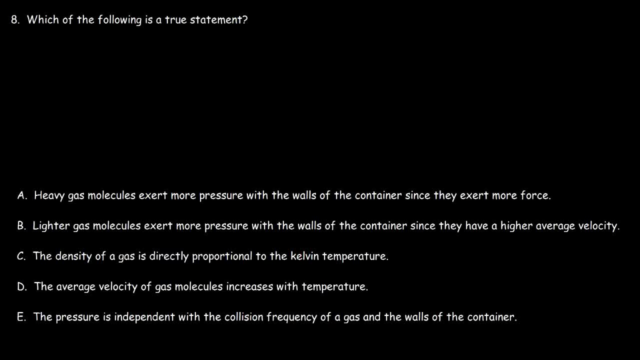 tend to move faster and so these two, they sort of balance each other out and it turns out that they exert the same pressure. pressure doesn't depend on the molar mass of a gas, so it doesn't really matter. if the gas is heavier, light the heavy gas particles and move slow and 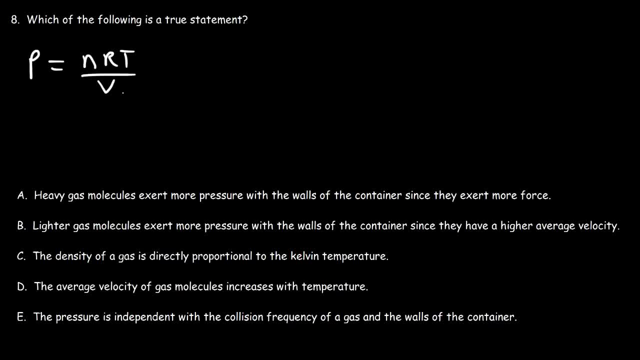 the light gas particles will move fast, and so it turns out that the average out to be the same. the average kinetic energy between heavy gas molecules and light gas molecules is the same. it only depends on temperature. so both A and B are false statements, even though lighter gas molecules will have a higher average. 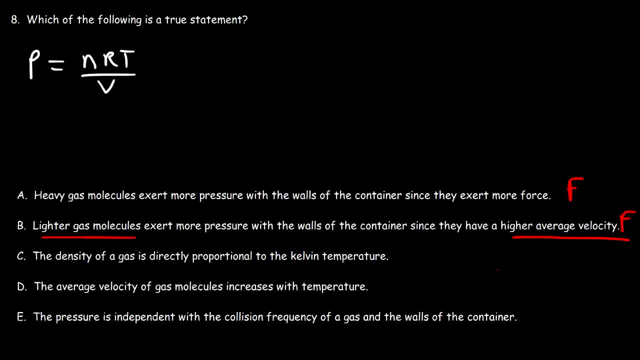 velocity, which would typically yield a greater pressure, the mass is less, and so if you have less mass, you have less force, even though you have, it's moving at a higher speed, and here there's more mass, which means there's more force, but the speed is less, so it turns out that the pressure is going to be the same, so 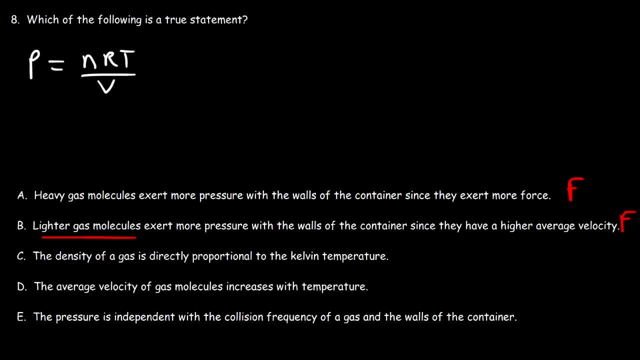 pressure does not depend on the molar mass of the gas. now what about the density? is the density directly proportional to the Kelvin temperature? density is equal to the pressure times the molar mass divided by RT. now notice that the temperature is in the bottom of the equation anytime you increase the temperature, you increase the pressure, you increase the pressure, you increase the denominator of a fraction. the value of the whole fraction goes down. so if you increase the temperature, the density of the gas will decrease. and it makes sense, because if you increase the temperature, the volume goes down and density is mass. divided by volume, so the mass of the gas will be the same. but anytime you increase the volume of an object, the density goes down, and so temperature leads to an increase in volume, according to Charles law, and that leads to a decrease in the density of the gas. so the density is inversely proportional. 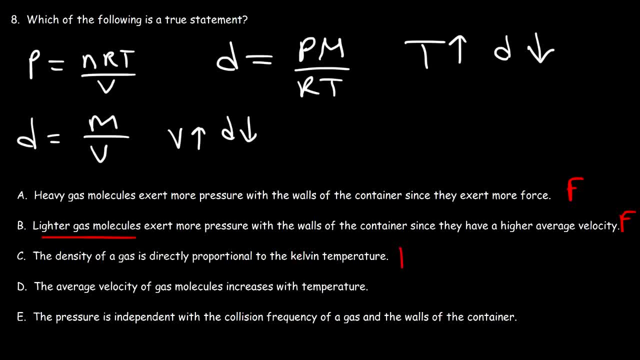 to the Kelvin temperature, which means C is a false statement. now, density is directly related to pressure and molar mass. if you increase the pressure of a gas, the density of that gas will increase, and if you increase the molar mass of a gas, the density will increase. 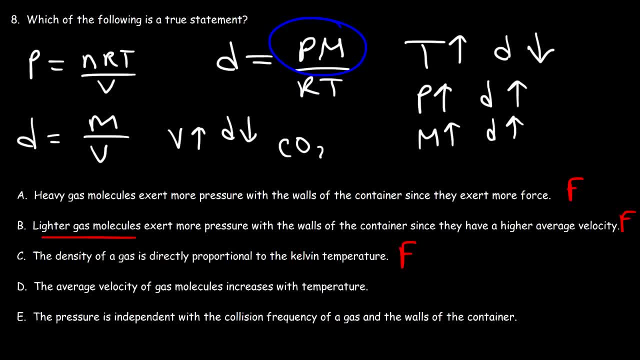 so if you compare two substances like co2 versus neon, where everything else is, else is the same, CO2 will have a higher gas density because it has a higher molar mass. Now what about D? The average velocity of gas molecules increases with temperature, Is that? 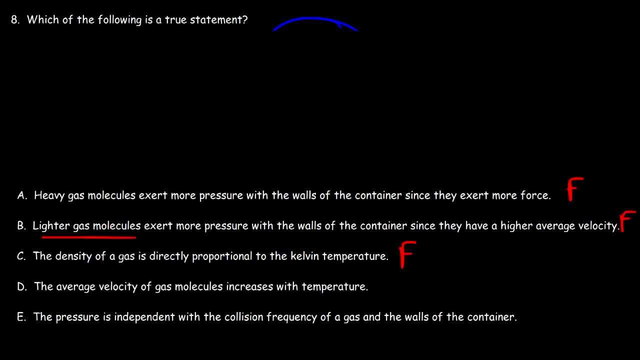 true or false. So recall this equation: The root mean square velocity is equal to the square root of 3RT divided by the molar mass. So if you increase the temperature, the average speed will increase. So D is a true statement. If you increase the molar mass, the speed will decrease, As we said. 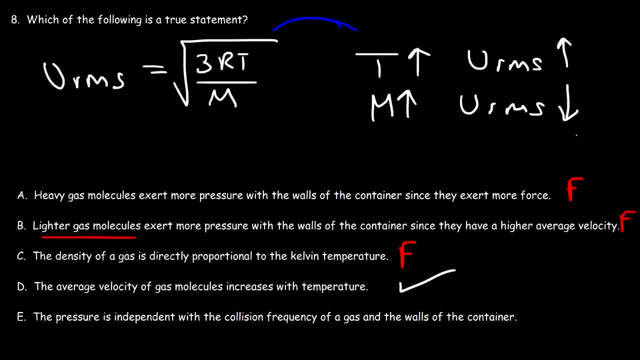 before. heavy gas molecules move slower. lighter gas molecules move faster. Now what about E? The pressure is independent with the collision frequency of a gas and the walls of the container. That's a false statement. The pressure depends on the number of collisions between the gas particles and the walls of the. 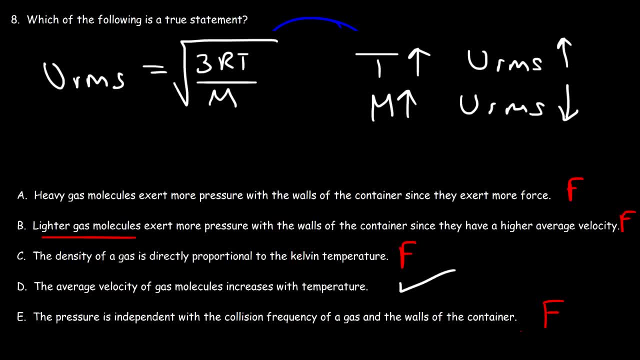 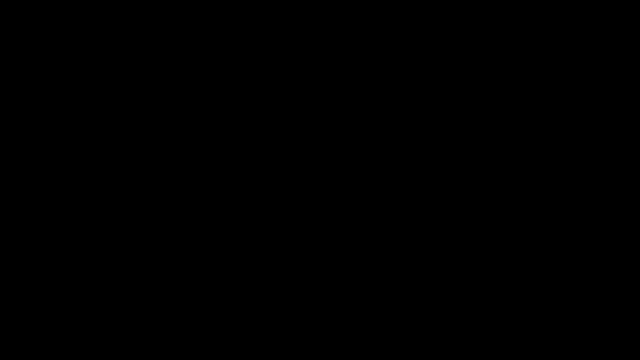 container. As the collision frequency increases, the pressure increases. Now let's go over some free response questions. Not only do you need to know the gas laws, but you need to understand why they work the way they do. So let's start with Boyle's law. If we decrease the volume we know 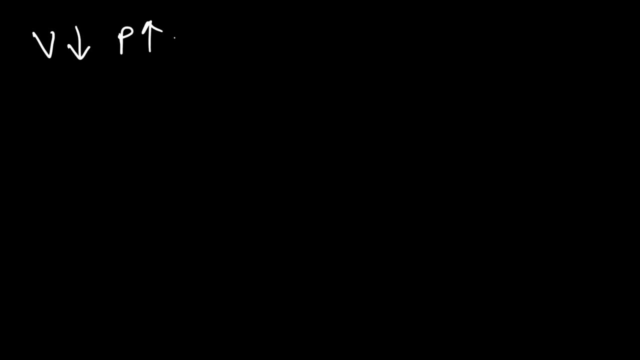 that the pressure will increase. The question is: why does that happen? Go ahead and explain it. Feel free to pause the video and write out an explanation if you want to. So let's say, if we have a container this large and it contains: 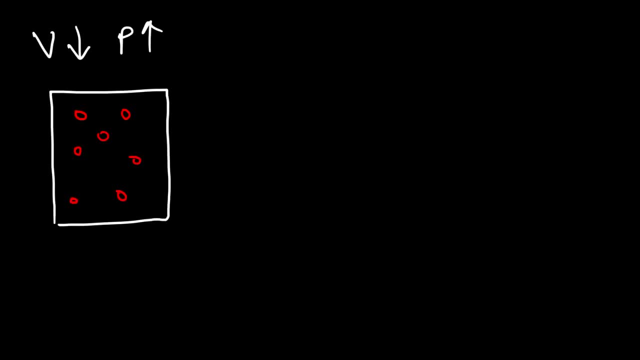 some gas particles. Now, if we reduce the volume, why does the pressure increase? When dealing with pressure, you need to describe it in terms of the amount of pressure. So let's say that we have a container this large and it contains some gas particles. 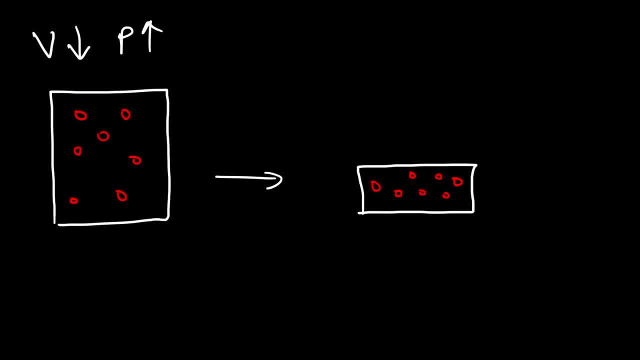 terms of the collisions. As you reduce the volume, notice that there's less space, and so those particles will collide more frequently with the walls of the container, and that's why the pressure goes up in the case of Boyle's Law. So make sure you understand that When you reduce the volume, 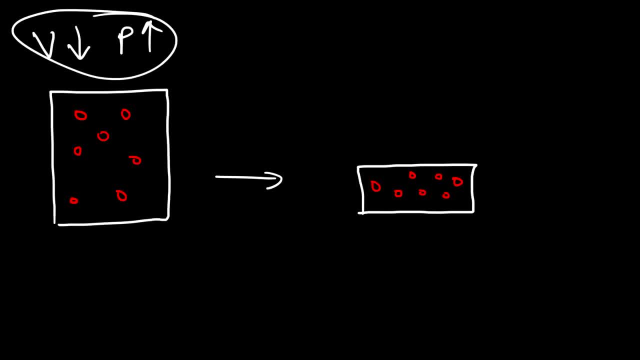 the collision frequency goes up. As the particles collide more often with the walls of the container, the pressure goes up. Now the next thing we need to talk about is Gay-Lussac's Law. Actually, let's go over Avogadro's Law first. If we increase the moles, the volume increase. 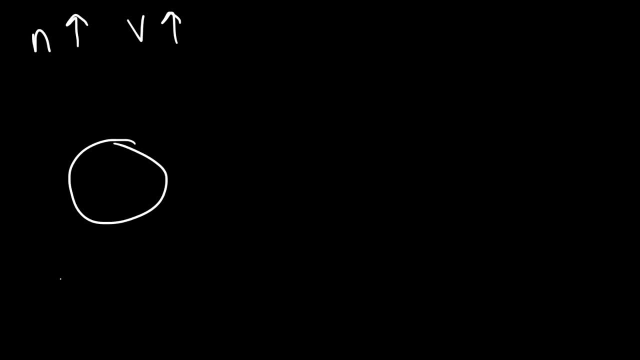 So let's say, if we have a balloon and there's only one mole of gas, If we add more gas, we know the balloon will expand. The question is why? Why does the balloon expand? Well, for one thing, as you increase the number of moles of gas, particles initially. 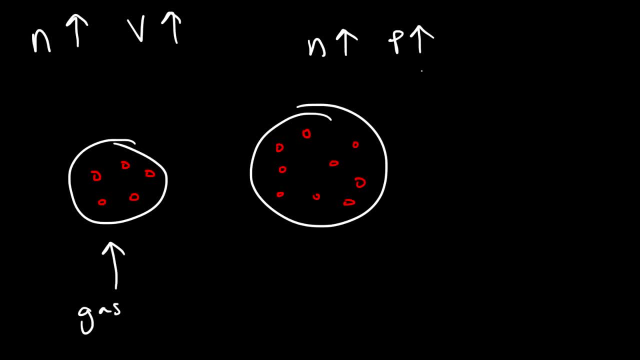 the pressure is going to go up. So I'm going to have to draw this visually. So, before the volume increases, the instant you add more gas particles you're going to have more collisions between the gas particles and the inside wall of the balloon. So the pressure goes up. Now, let's say, before that happened. 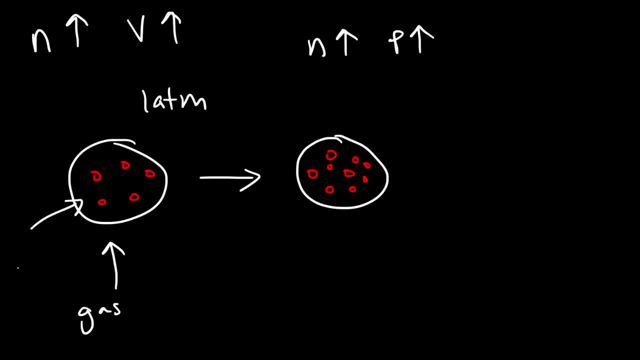 the outside pressure is 1 atm, The pressure on the inside is also 1 atm, So the volume doesn't change. But as soon as you add more gas particles in the balloon, the pressure is going to increase. The inside pressure might be 2, the outside pressure might be 1. And so the forces on the inside exceed. 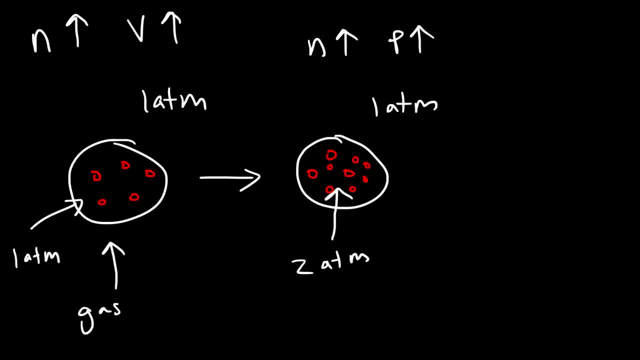 the forces on the outside And, as a result, due to this lack of equilibrium, the balloon is going to expand And it's going to expand until it reaches equilibrium. So you're still going to have more gas molecules Inside this balloon, But the volume is going to double to bring back the pressure down to. 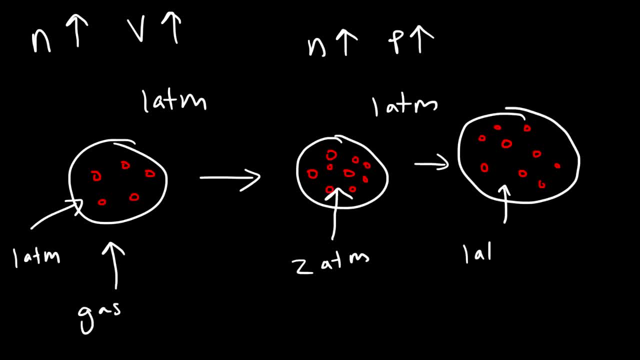 1 atm, So the volume will no longer increase when the inside pressure is equal to the outside pressure, And so that's why the volume goes up. So let's just review what we just said. As you increase the number of moles in a container, like a balloon, like a flexible container, 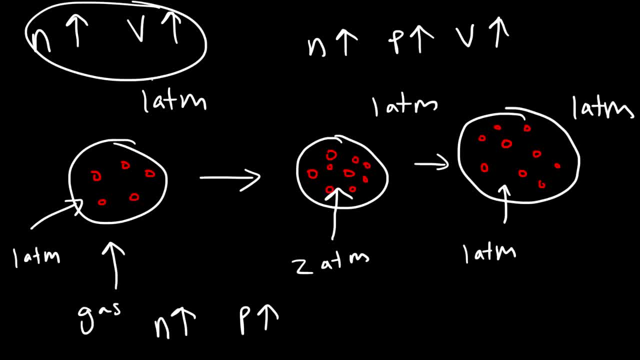 itultually, the pressure goes up, Going up from 1 to 2.. And as a pressure increases, the internal pressure exceeds the external pressure, And so the volume will increase. And, according to Borel's Law, as you increase the volume, the 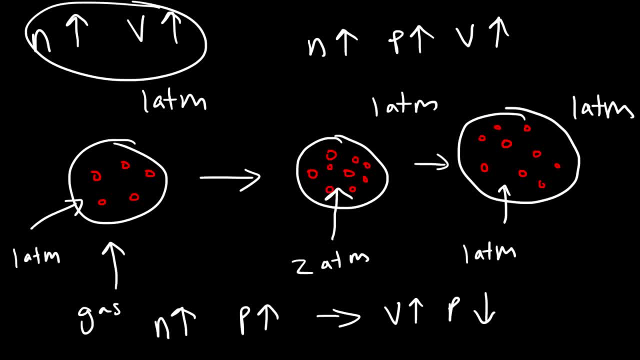 pressure will decrease. So the net result is that there's no change in pressure. The pressure goes up and then it goes back down, So the net change will be increased. change in pressure is 0. So as you increase the moles, the final result is that the 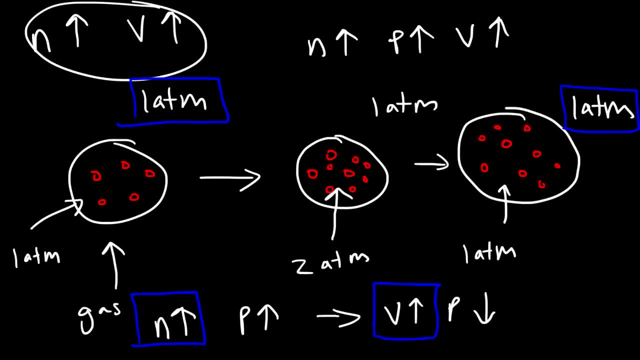 volume goes up. It goes up due to a change in pressure, but in the end the pressure goes back to its normal level. When the inside pressure is equal to the outside pressure, the volume will not increase or decrease. It's going to stay. 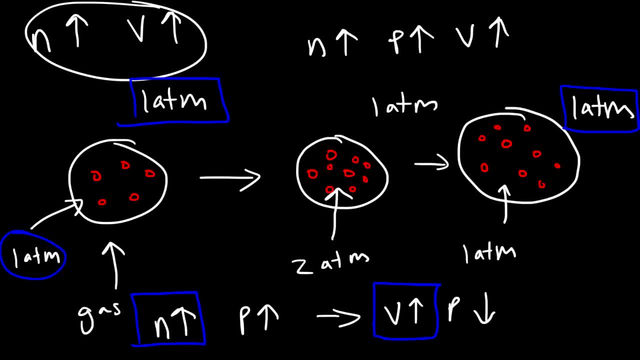 the same. When you increase the moles, the pressure goes up, which causes the volume to go up until equilibrium is re-established and then the pressure goes back down. So the net result is: as you increase the moles, the volume will. 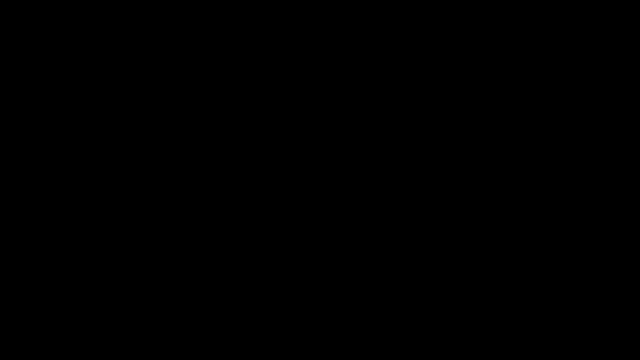 increase. So that's Avogadro's law. Now what about Gay-Lussac's law, where, if we increase the temperature, the pressure will increase? So let's say, if you have gas particles in a container where the volume is fixed and the temperature is 300 Kelvin, what's? 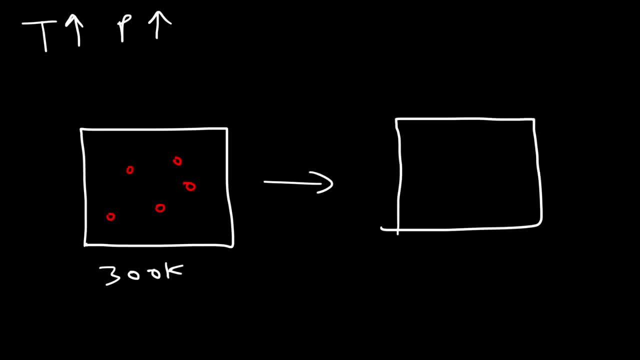 going to happen if you increase the temperature to, let's say, 500 Kelvin Now, the number of particles will not change. However, we know that the speed- the root mean square velocity- is dependent on the temperature. So as you increase the 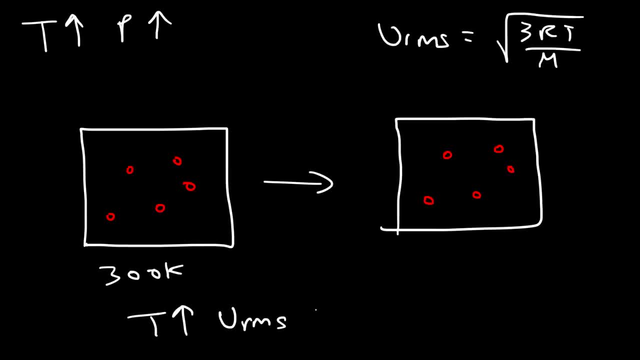 temperature, the average speed will increase, And so the particles will be moving a lot faster. So if they're moving faster, they will collide more frequently with the walls of the container, And if you can increase the collision frequency, then the pressure will increase, And so 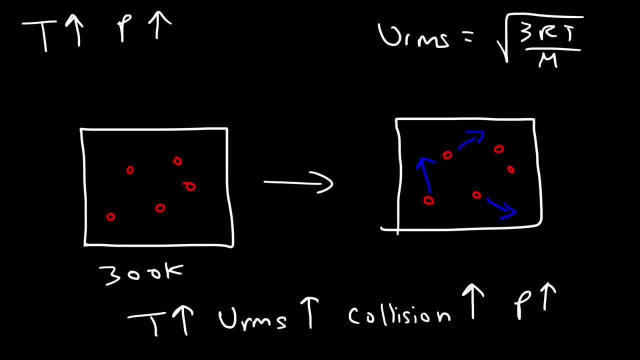 that's how an increase of temperature will lead to an increase in pressure. The speed of the molecules will increase. they will collide more frequently with the walls of the container, which leads to an increase in pressure. Now the last one is Charles' law, which is a combination of the other laws. As the temperature goes up, 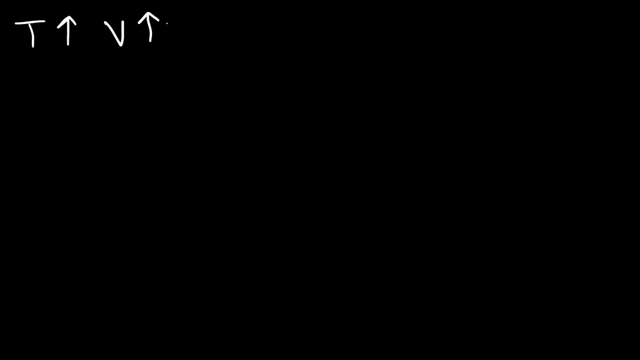 the volume goes up. Now let's talk about why. Let's use a balloon for this example. Well, if you increase the temperature, we know that the average speed of the molecules will increase And this will lead to a greater collision frequency And, as a result, the pressure will go up. So let's say, if we have a balloon and 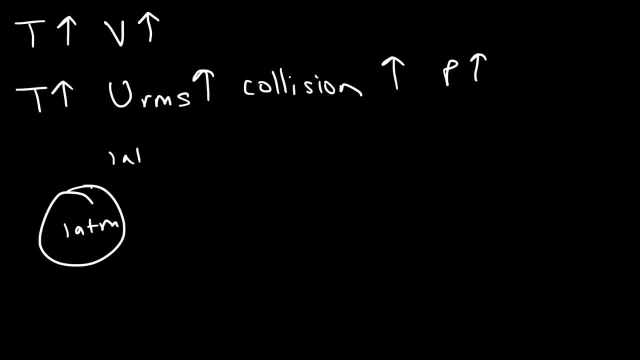 the inside pressure is one atm and the outside pressure is one atm at 300 Kelvin. Now as we increase, let's say, the temperature to 600 Kelvin, the molecules inside the balloon will be moving faster, And so instantly the pressure is going to. 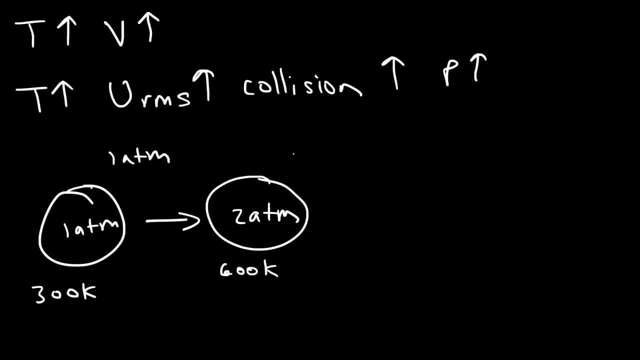 go up from one atm to two atm. Now, because the internal pressure exceeds the external pressure, the gases on the inside will exert more force compared to the gases on the outside, And so the balloon will expand. As it expands, the internal pressure will decrease And it's going to stop expanding. 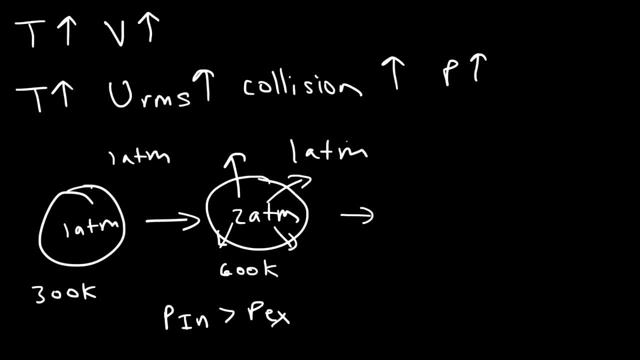 until the pressure is equal to the outside pressure. So it's going to continue to expand until the inside pressure is back to one atm. So once the inside and the outside pressure are equal, it will stop expanding. The volume will no longer change, And so that increase. 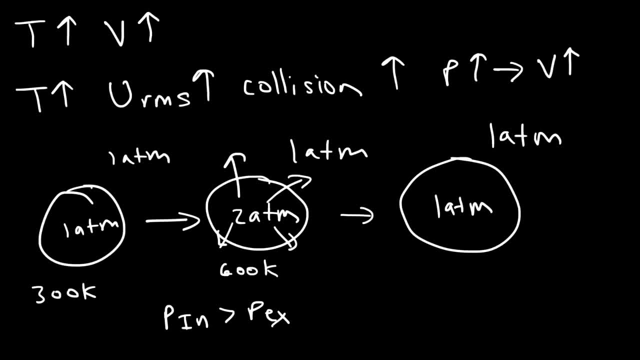 in pressure will lead to an increase in volume, which brings back the pressure back to one atm or to the atmospheric pressure. So this increase in pressure and then a decrease in pressure negates each other. So the net effect is that the pressure remains the same as we.